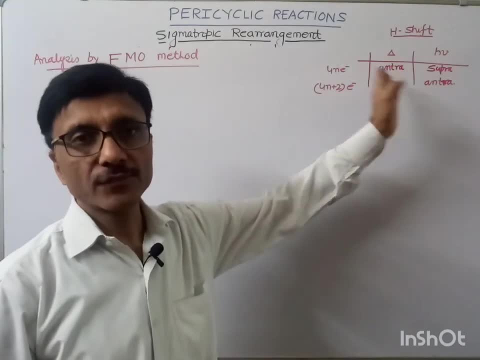 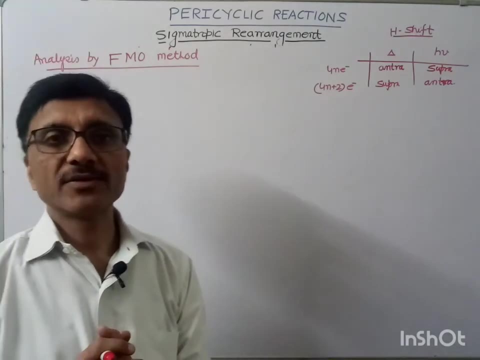 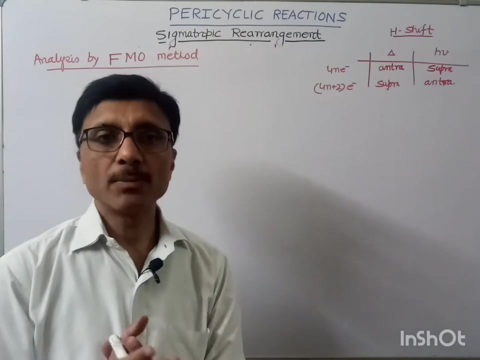 Now let us prove this selection rule by frontier molecular orbital method. We know that in frontier molecular orbital method we take two components. one component: we divide the whole molecule into the two components, and one is taken as HOMO, another is taken as LUMO, and vice versa. 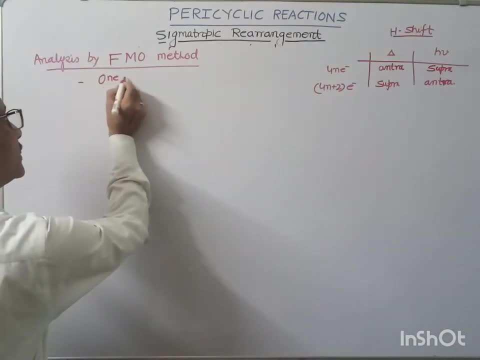 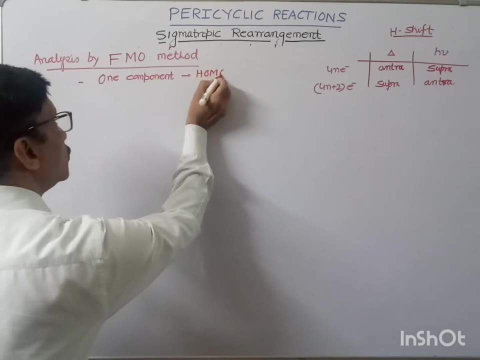 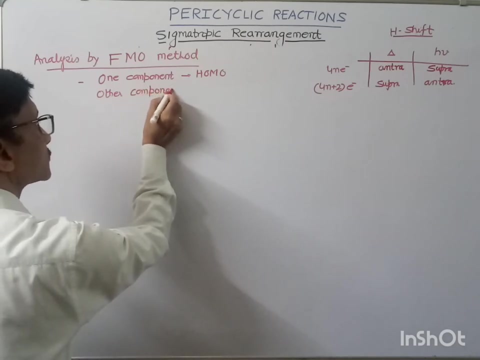 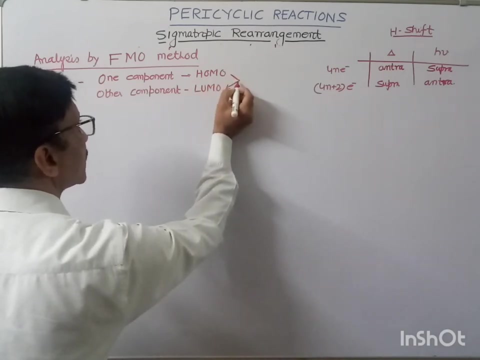 So here in FMO method, what we do, One component is HOMO, other component is LUMO. This is taken as LUMO or vice versa. we may take vice versa, either this one, this may be taken, this one or this may be like this: 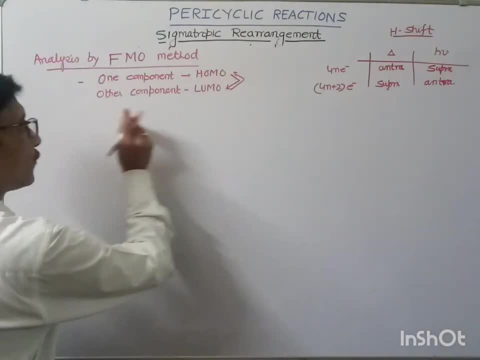 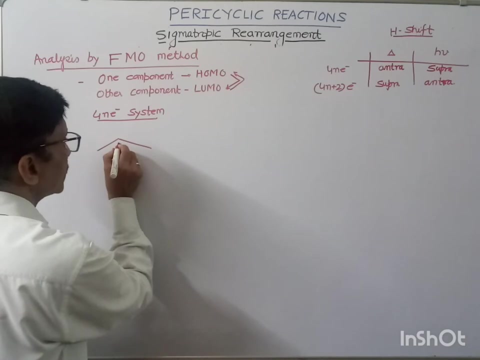 Okay, Now let us see for foreign electron system first. Okay, Now for foreign electron system. suppose, if we have HOMO, this is taken as HOMO. This is taken as HOMO, This is taken as HOMO. 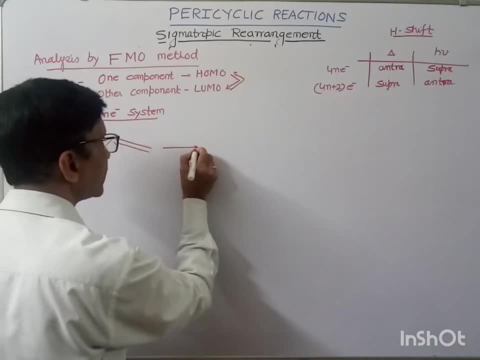 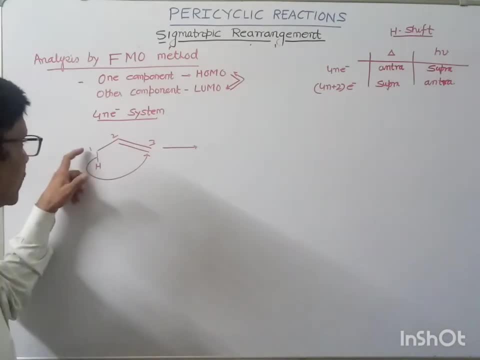 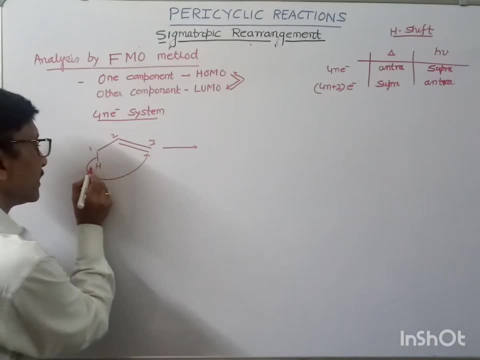 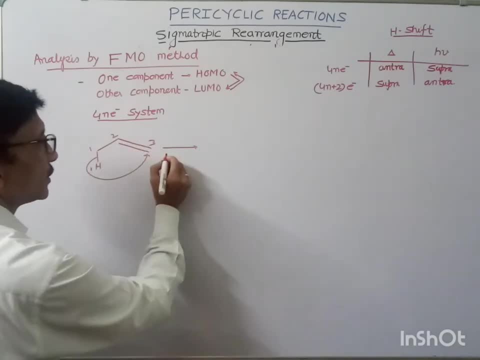 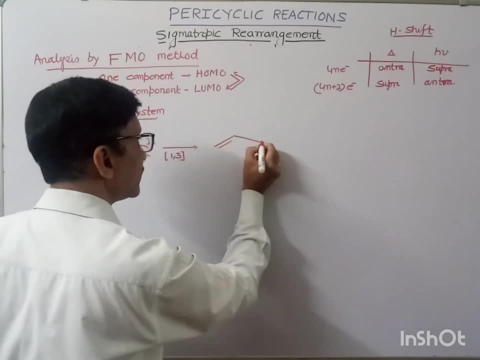 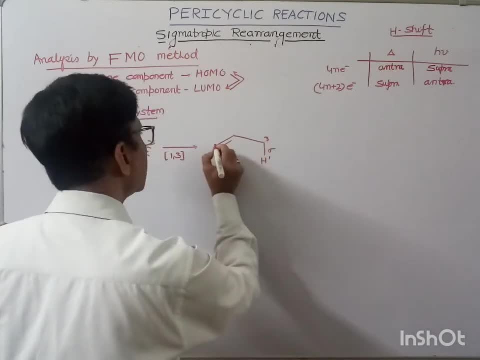 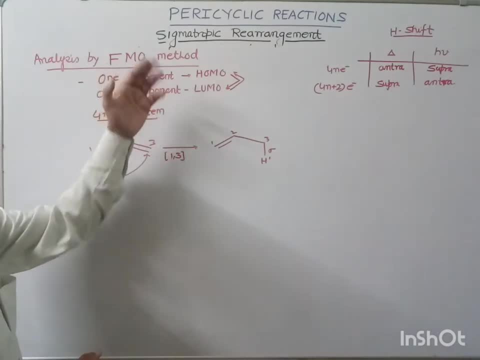 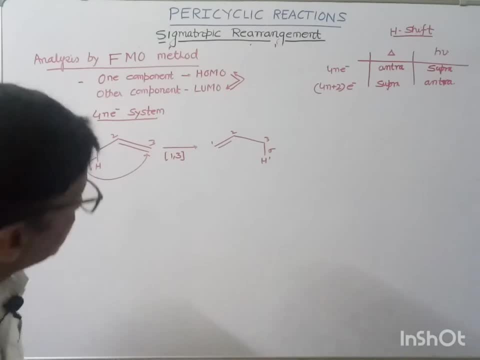 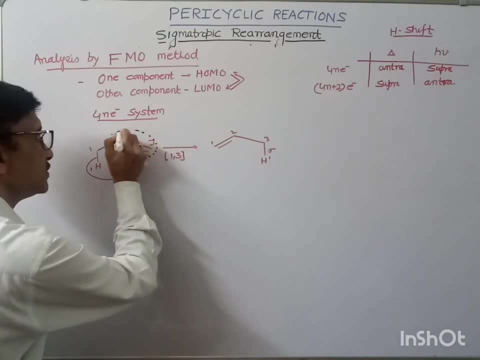 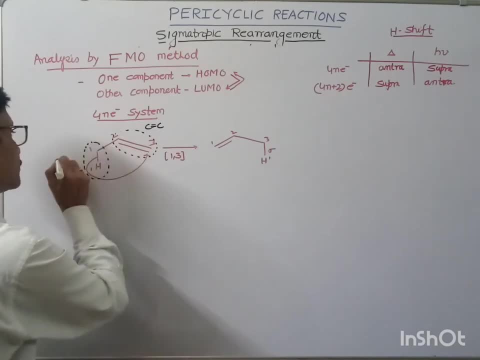 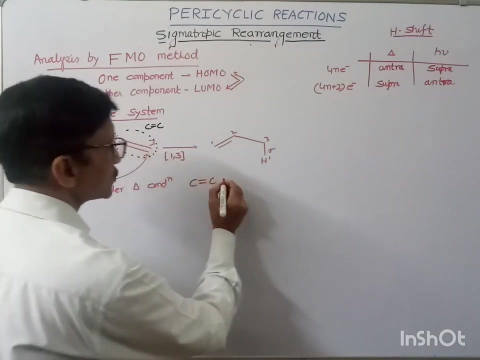 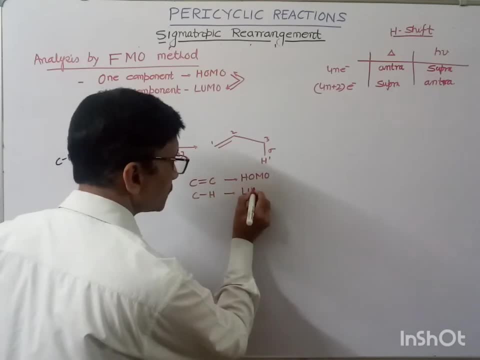 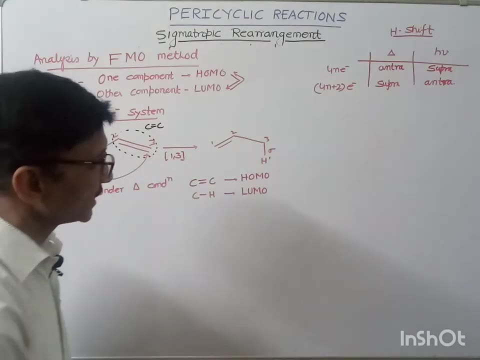 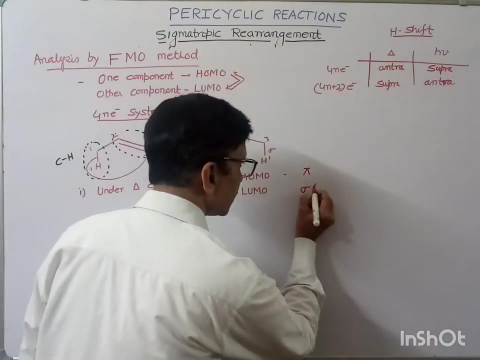 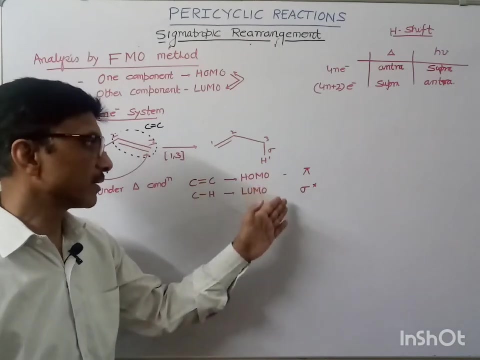 Sigma bond is taken as LUMO. so homo of this alkene type of system, ethene system, that is all of you know. this is our PI- is the homo and LUMO, for this is Sigma star is the LUMO or otherwise, we may take in a another. 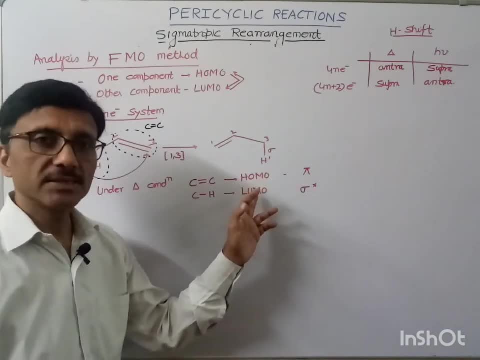 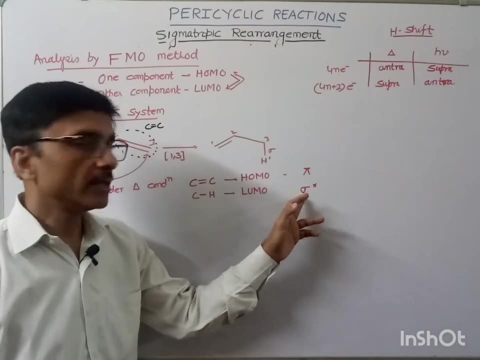 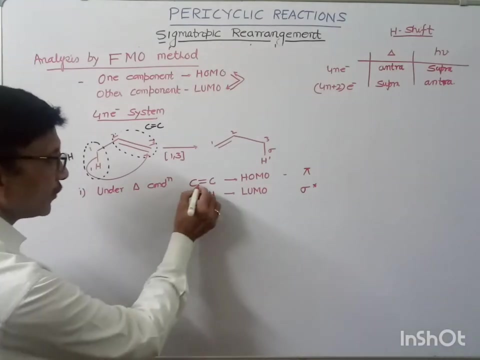 opposite manner also. this may be taken as LUMO, this may be taken as homo. if I take it LUMO, then it would be PI star. if I take homo, this would be Sigma. then result: that come out to be same in both cases. that will come to be same now if 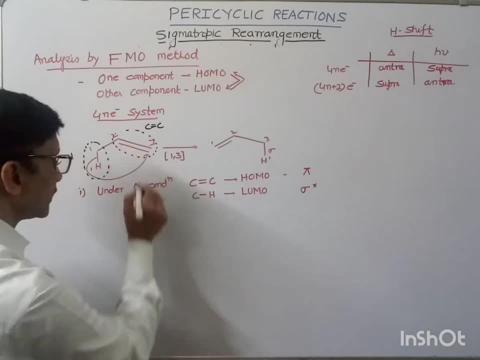 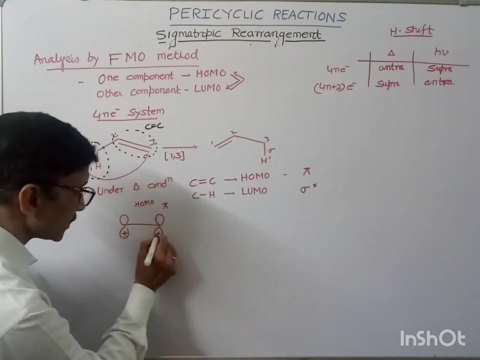 this is one, this is homo, then what I should write: suppose this is our C, single bond C, C, double bond C, and if this is our homo, this is homo, that is PI, and then it would be plus, plus, and this is minus, minus, plus. this is C, double bond C. now it is attached to this. 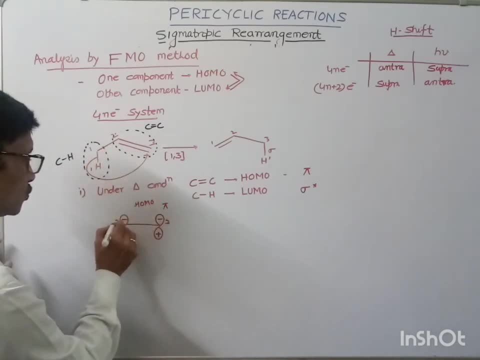 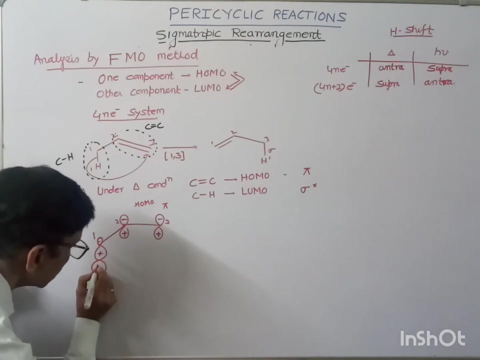 bond. this is suppose at three, this is two and this is our one. and now CH bond. CH bond is LUMO of CH bond, so LUMO of CH bond plus minus, and this is our CH bond. this is H plus minus, so this represents the Sigma star. this represents the Sigma star. 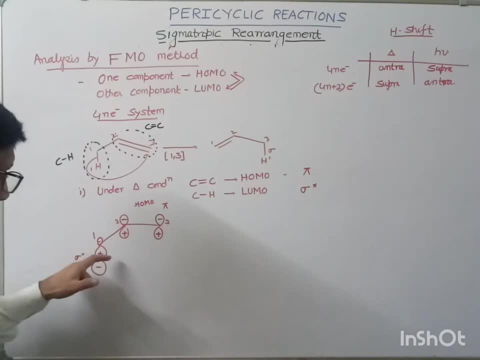 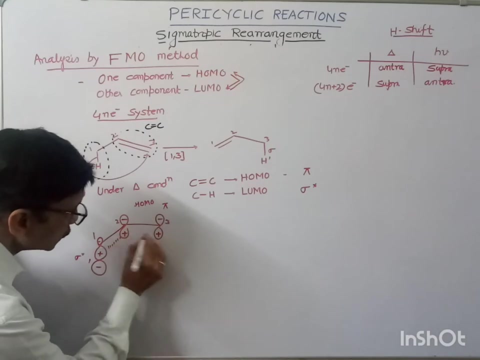 one, one, one one. so this bond will break, this bond breaks and it will form bond with this third carbon atom. now, if you will see in this case, then here the interaction, if you see the superficial interaction- sorry, if you see the superficial interaction- then this will interact with this lobe and this lobe. 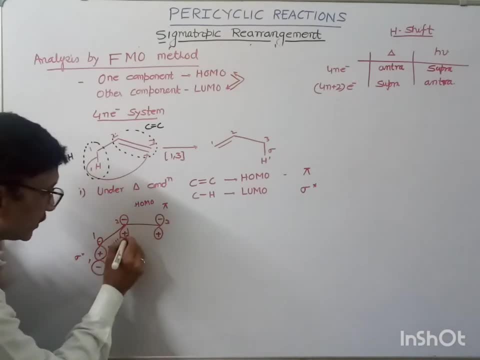 these are the two same side lobe of ethene system. it will interact with the. this is CH and Sigma bond bonding interaction over here and this will also form a bonding interaction over here. sorry, this is forming the anti bonding interaction. so superficial interaction is disallowed over here. so supra is. 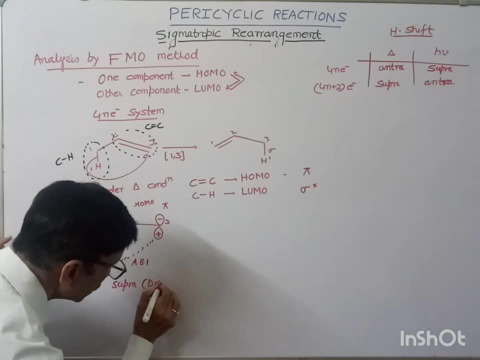 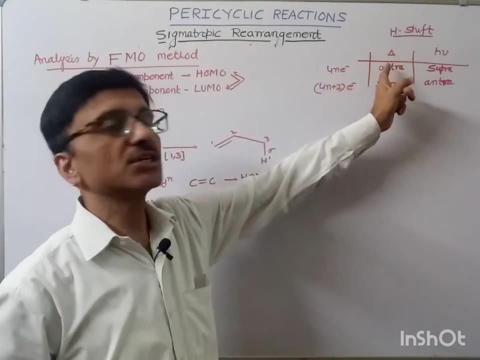 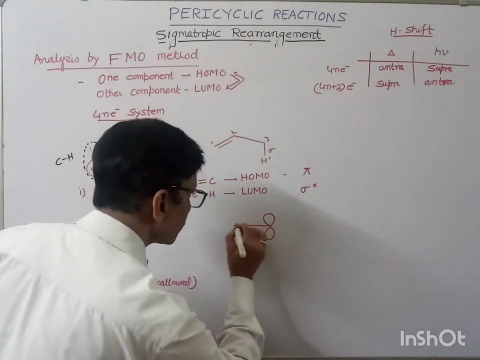 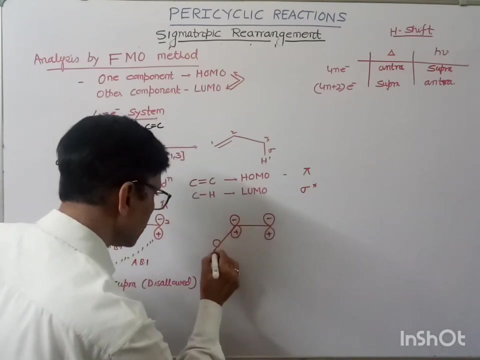 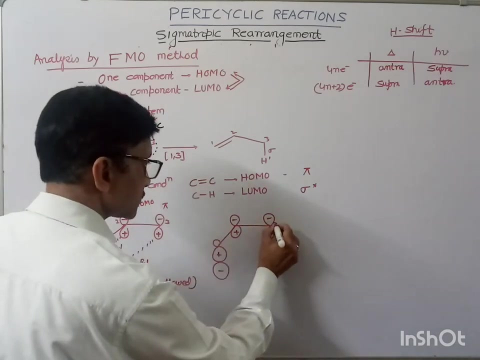 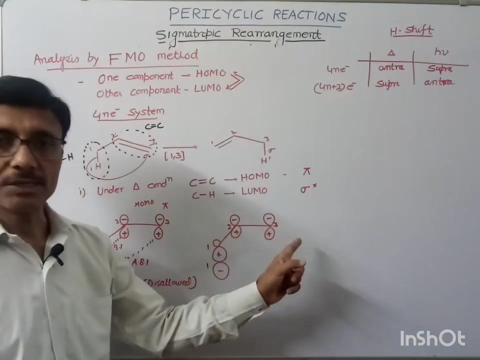 disallowed supra is disallowed under thermal condition. so what is the rule? under thermal condition, entra is allowed. let us see for entrafacial interaction and the entrafacial interaction. okay, so again, this is third, second, first and this will also first. first will form our bond with third. so interfacially means: 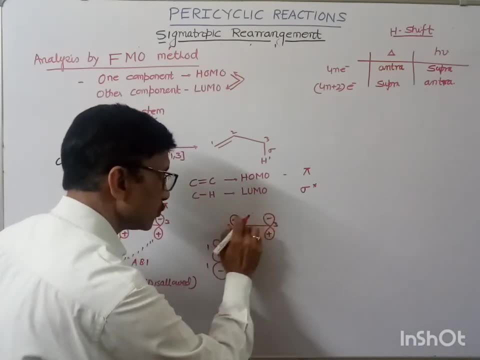 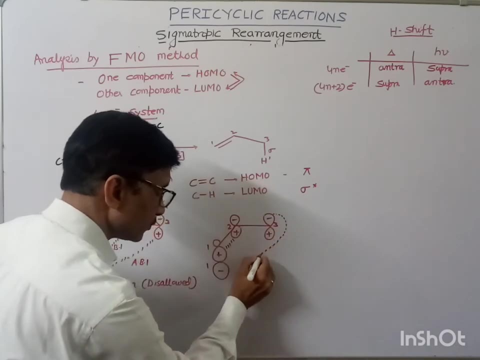 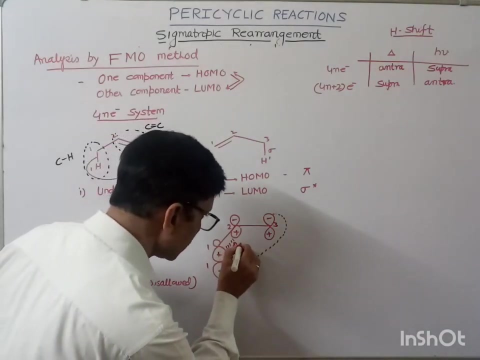 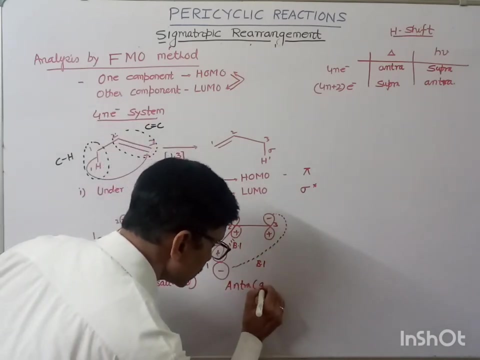 interfacial, different opposite side lobe that will interact. if this is in this lobe, then another interaction would be. this would be the another interaction. so this is interfacial interaction. so here this is bonding interaction, here also it is the bonding interaction. that's why entra is allowed. entra is allowed here under: 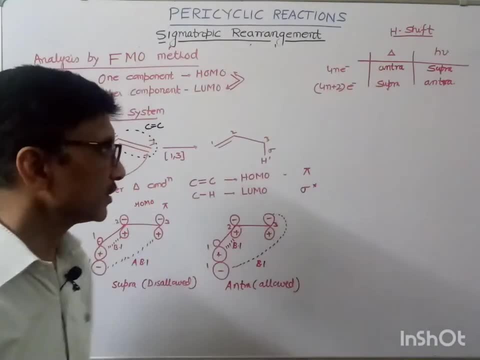 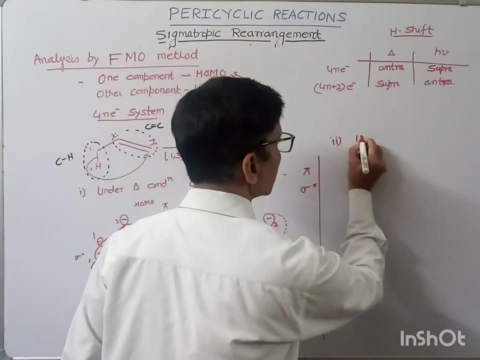 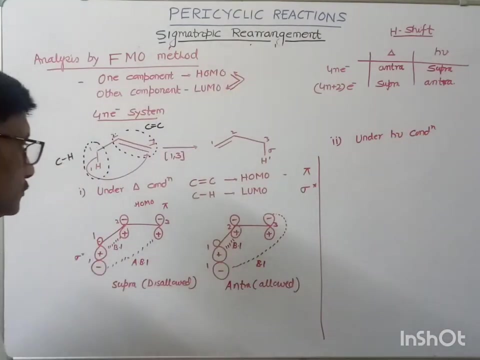 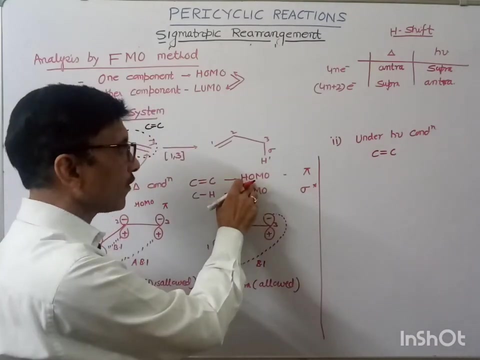 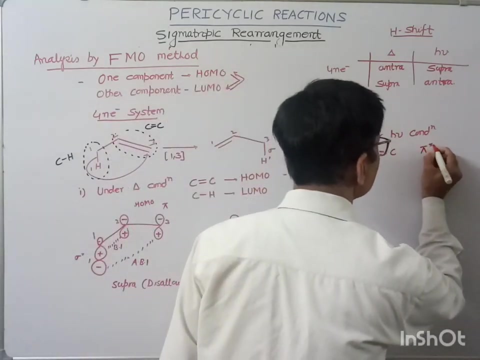 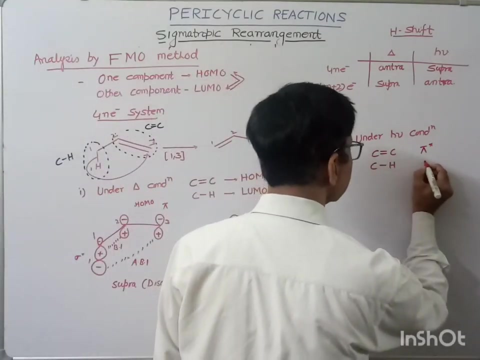 thermal condition. entra is allowed. that we have seen now under photochemical condition. if you see under photochemical condition now C, C, C, double bond, C bond, that would be homo of C, double bond, C bond under photochemical condition, that would be pi star. that would be pi star and LUMO would be. LUMO would be Sigma star only. 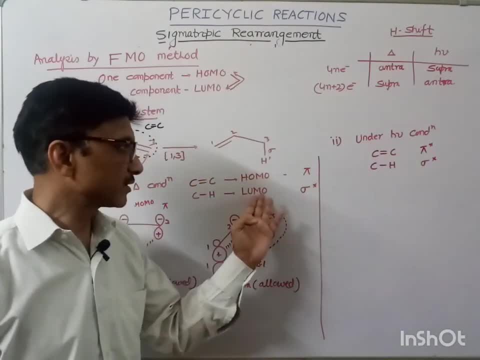 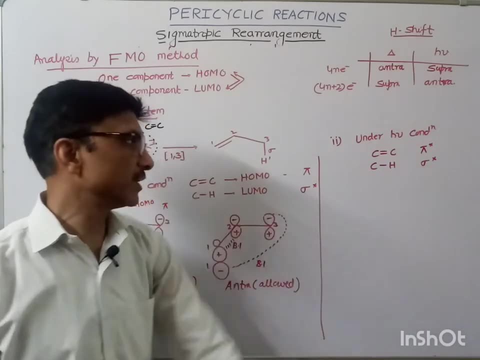 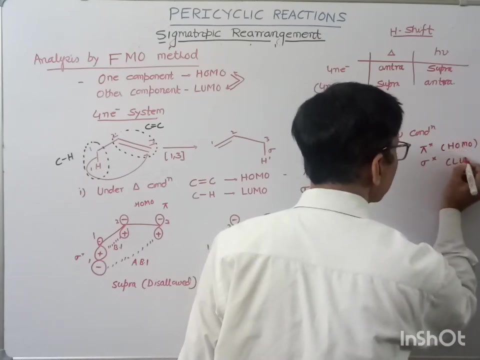 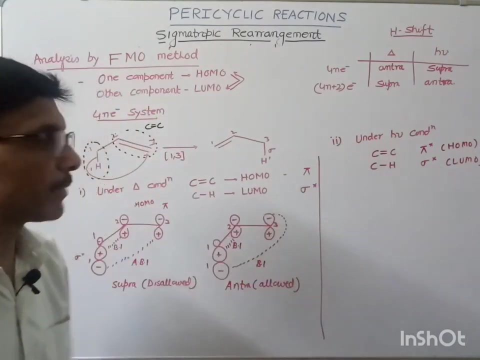 under photochemical condition or under thermal Sigma star, as well as under photochemical condition also, the homo would be, the LUMO would be Sigma star. so this is our homo under photochemical condition and this is the LUMO under photochemical condition. now, so C? double bond, C is pi star. c double bond, c is pi star. 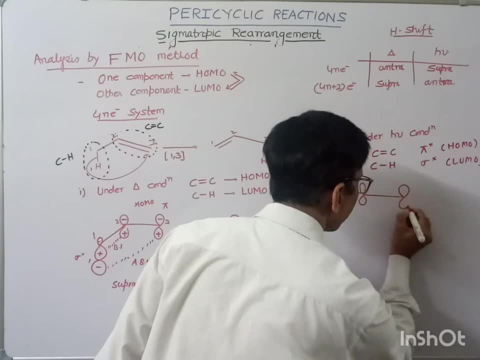 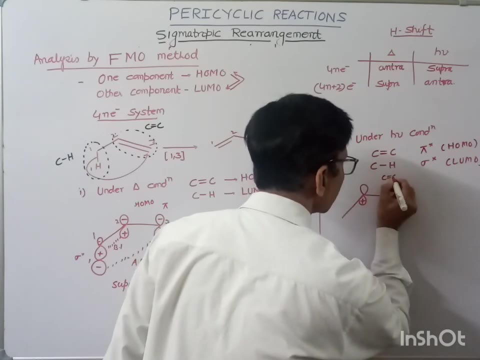 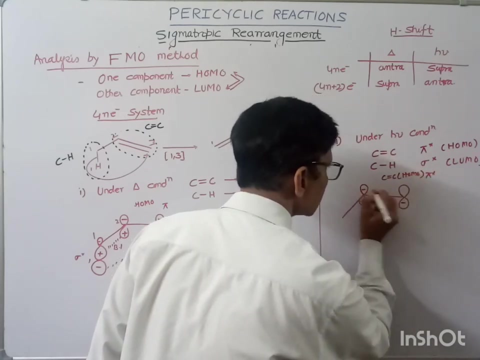 pi star means plus, minus. so this is our homo C double bond C: homo pi star. so I should write Pi star over here: plus minus. this is minus, there will be plus now. this is our homo homopistar, correct. but we have to write pi star over here now. this is our homo. now, this is our home. now this is our homo. plus or minus it multiply. this is the homo. homopistar live with us in the millionile phase world program. here is Slide and let us acknowledge here: homopistar live with us in the millionile phase world programas. you see it is indescribable. help you a is well that I can do, nonounてh Gordon to find out. 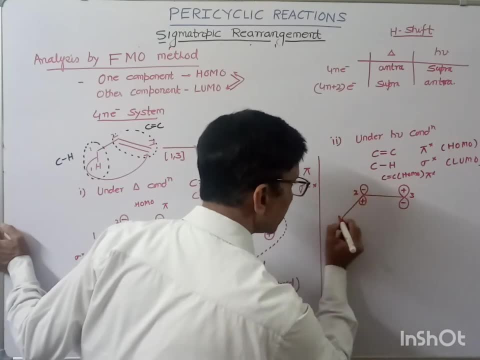 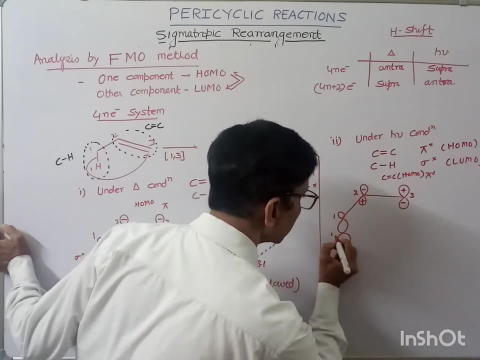 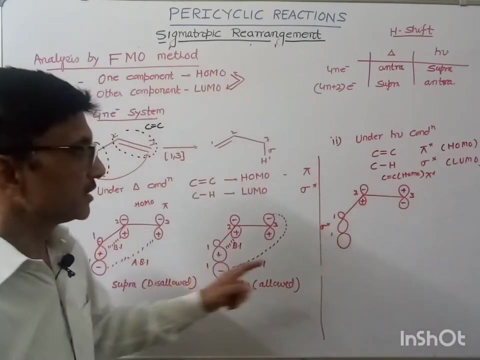 our third carbon. this is first second carbon and here this is our first carbon. First carbon is attached to one of the hydrogen and this is first one hydrogen. So this is sigma star. This should be sigma star, Cn should be sigma star. So sigma star means plus minus, Sigma star means 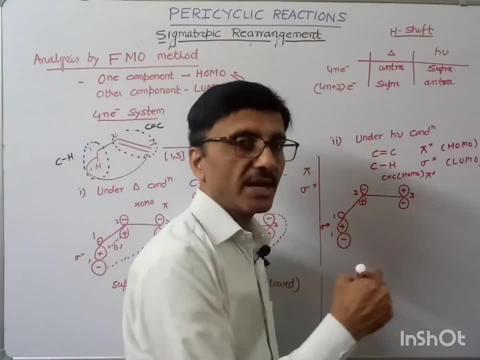 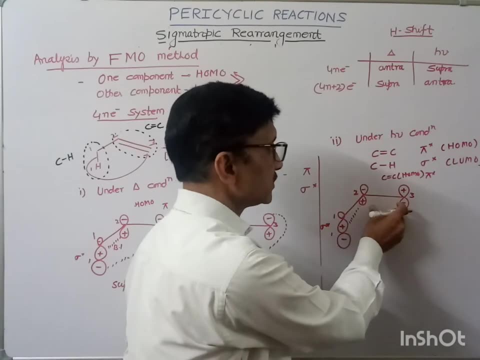 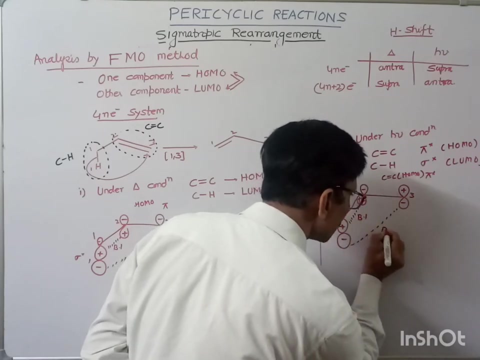 plus minus Now interact. Let us see the interaction in a suprafacial manner. So if you see, suprafacial means same side lobe of this C, level 1 C, that will interact, and same side lobe and you can see the bonding interaction Here also bonding interaction. So supra is 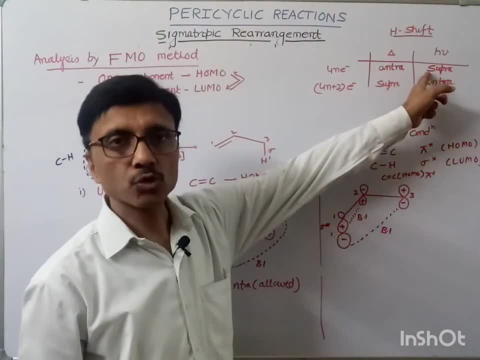 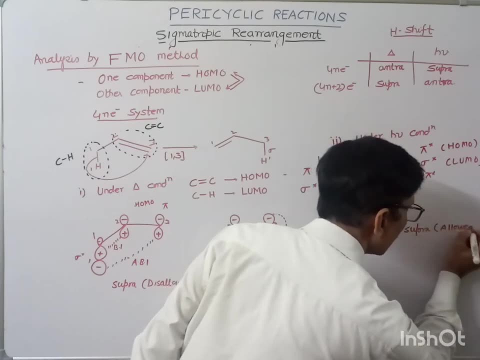 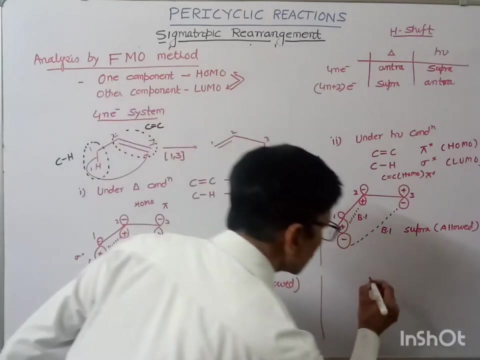 allowed under photochemical condition. Supra is allowed under photochemical condition. It is allowed. If you want to see under in ENTRA, then ENTRA will not be allowed under the photochemical condition. So let us see whether ENTRA is allowed under photochemical condition or not. 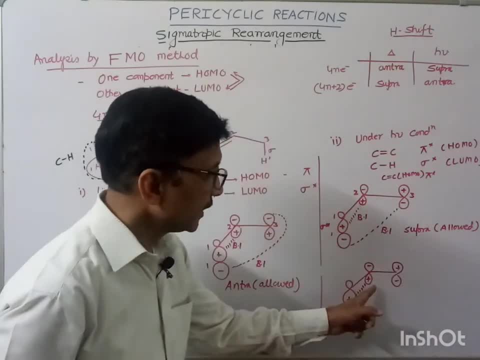 Okay, Now, now interact. interaction will be from the opposite lobe- Opposite lobe is allowed under the photochemical condition. So let us see whether ENTRA is allowed under the photochemical condition or not. Now this opposite lobe will interact. Now this: 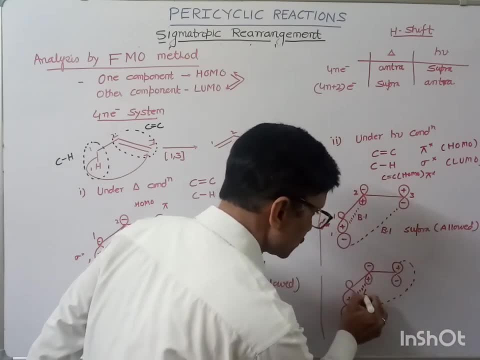 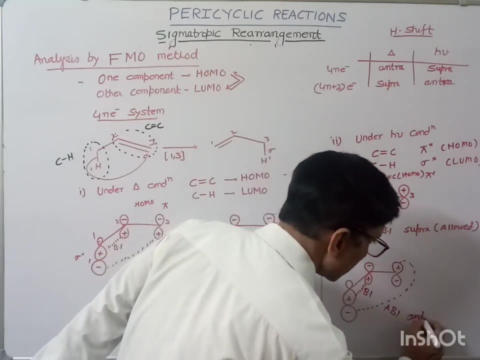 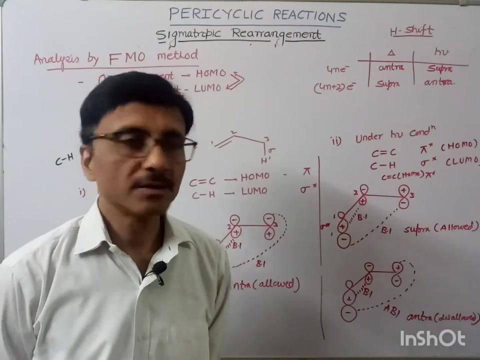 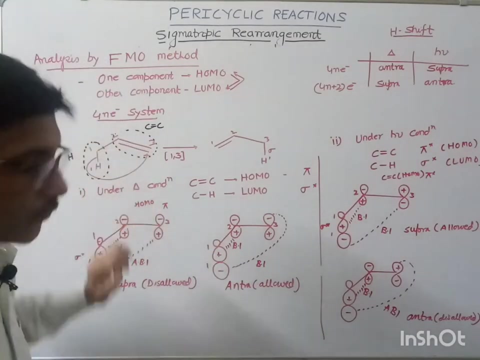 opposite lobe will interact. So this is bonding interaction, This is anti-bonding interaction and this is disallowed. so ENTRA is disallowed over here, Clear. So this is the case for 4n electron system. Now, if you will see, for 4n plus 2 electron. 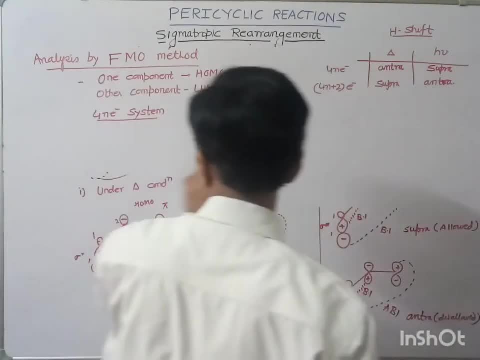 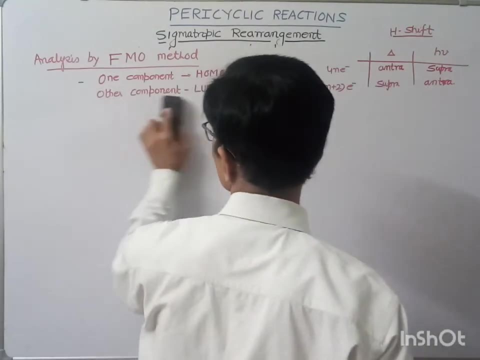 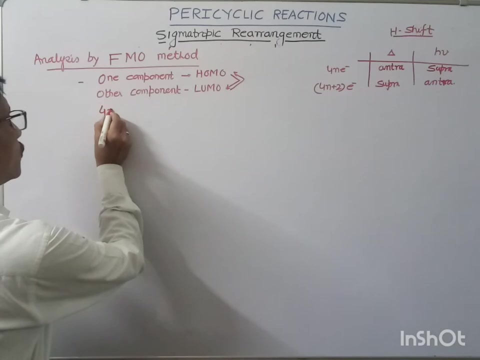 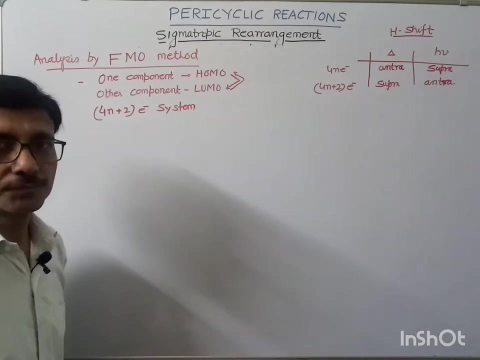 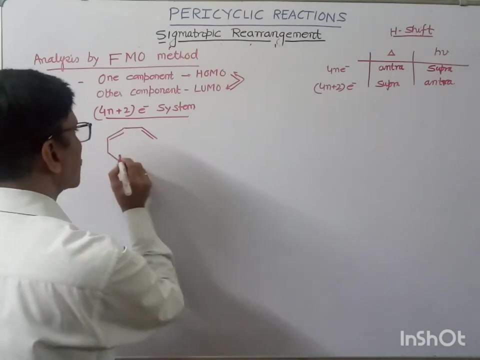 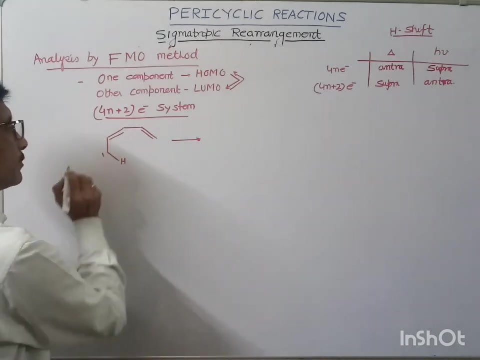 system. Now let us see for 4n plus 2 electron system. 4n plus 2 electron system Now. So first of all give the numbering. Lylic carbon is given number 1, 2, 3,, 4, 5.. 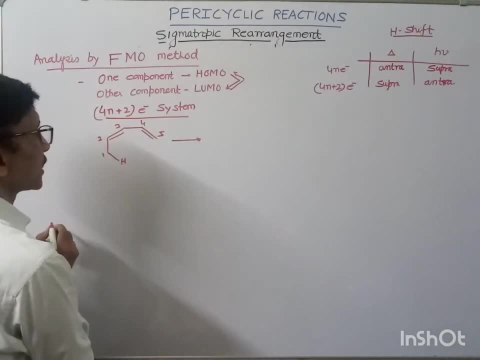 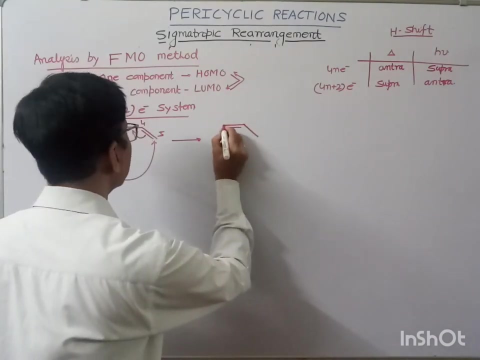 Atom which is attached to a lylic carbon atom is also given number 1. This sigma bond will break. as it gains the energy, Such kind of migration will take place. And here, single bond, double bond, single bond, double bond. And here the migration is taking place at the 5th position. 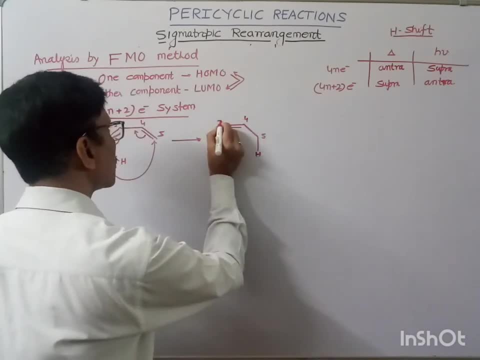 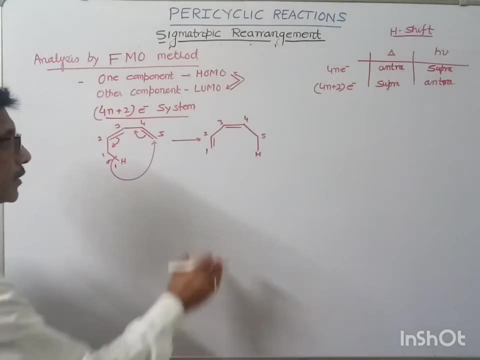 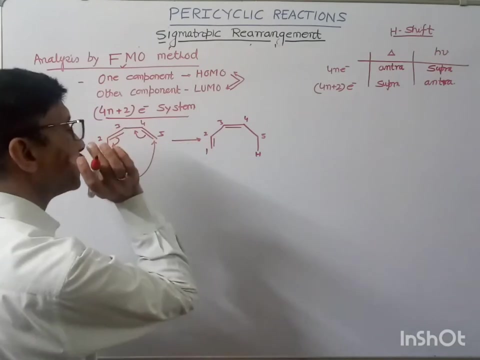 This hydrogen is coming at the 5th position, 4th, 3rd, 2, 1, like this: Ok Now. so if you want to see this rule, then by FOMO method. So one component is taken as the one component is taken as the HOMO. 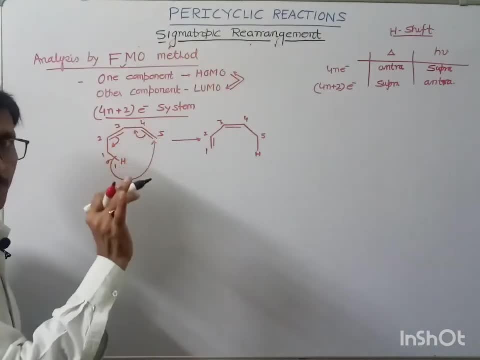 Another component is taken as the LOMO. So in here two component, How you can divide two component. This is one of the component And this is the other component, CH bond. So two component are. one of the component is butadiene. 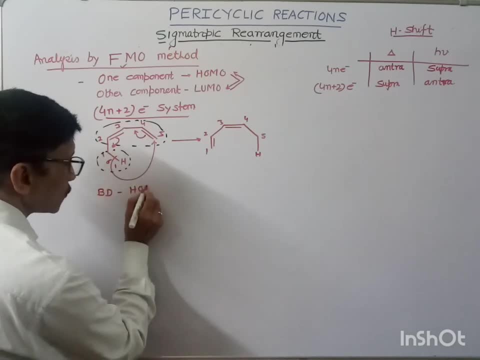 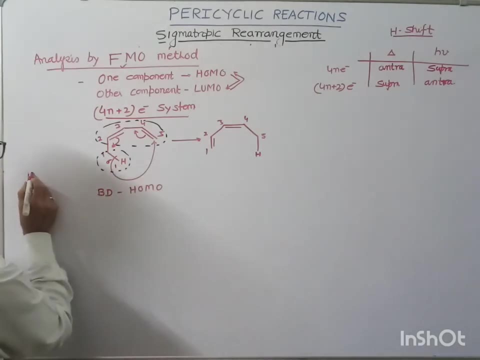 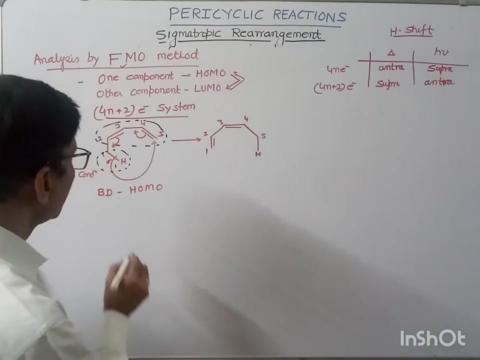 Butadiene is one of the component which I may take it as HOMO, The HOMO of butadiene, under thermal condition, So first of all under thermal condition. Under thermal condition Butadiene is HOMO and CH single bond is. I will take it as a LOMO. 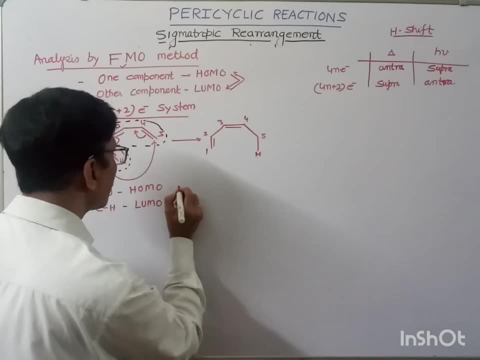 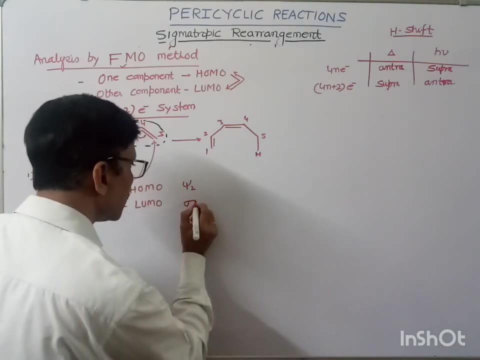 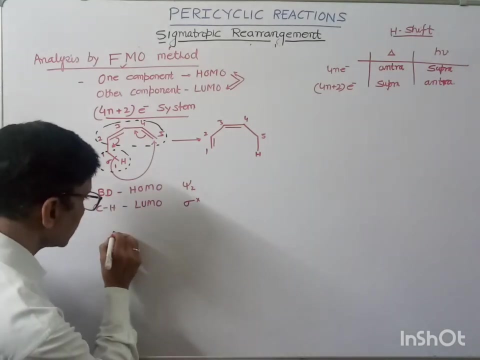 So if HOMO is HOMO of, butadiene is psi 2. And CH, that is sigma star, is the LOMO for this CH bond. Ok, So now let us see how we can show it. So this is the four orbitals of this butadiene. 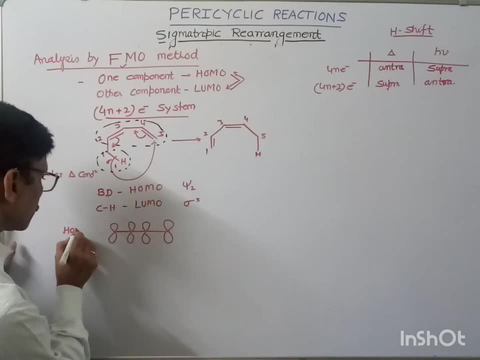 And psi 2, that is HOMO of this butadiene, I should write: And that is psi 2.. That is psi 2 means even molecular orbital, And for even molecular orbital, what I have told you, The opposite lobe, that should have the different sign. 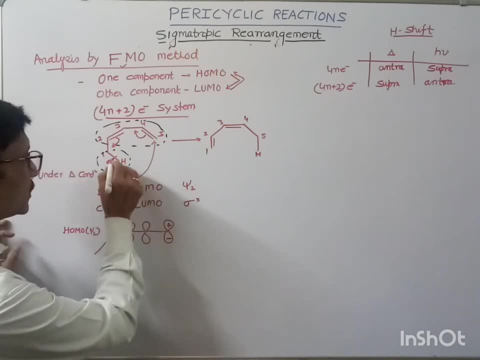 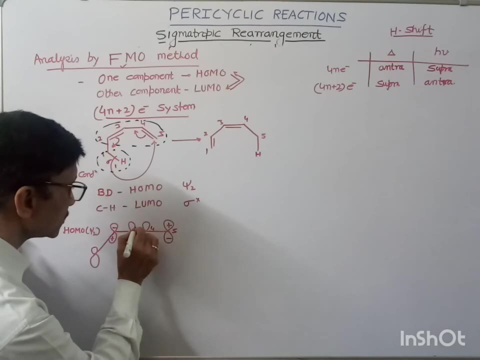 Now this interacts with. this is our CH bond, So this is our 5.. This would be 4.. This is 3.. This is 2.. This is 1. And positive and LOMO, Because this is LOMO, then this is positive, negative. 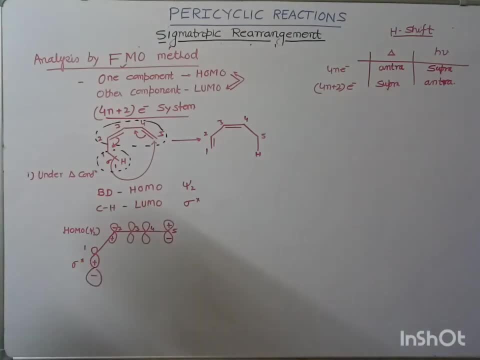 This is sigma star. Now let us see the interaction in a first superficial manner. So, in a superficial manner, this interacts with this one, And this interacts with this one And, as you can see, here, bonding interaction, Here also bonding interaction. 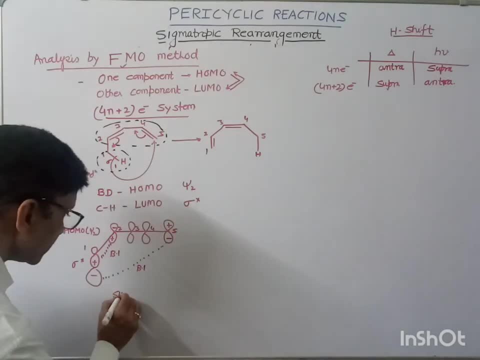 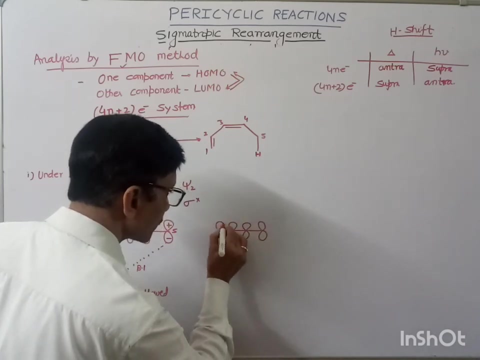 That is why. that is why this is supra is allowed. Supra is allowed. Now, if you will see for entra whether entra is allowed, No, entra is not allowed, Entra is not allowed. You can see Again: positive this is negative. 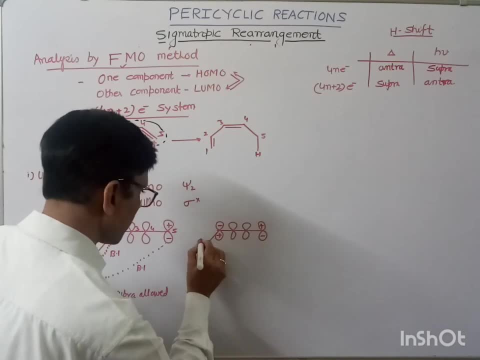 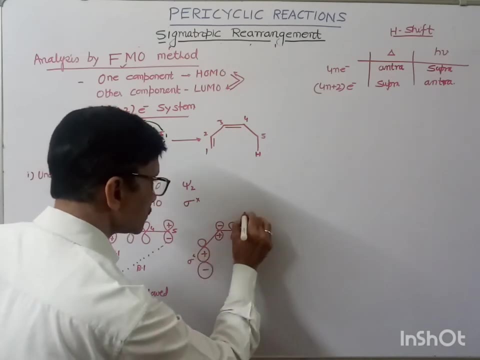 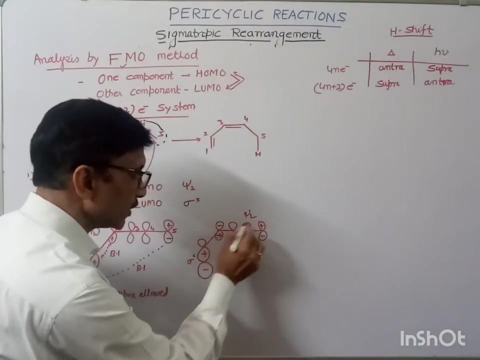 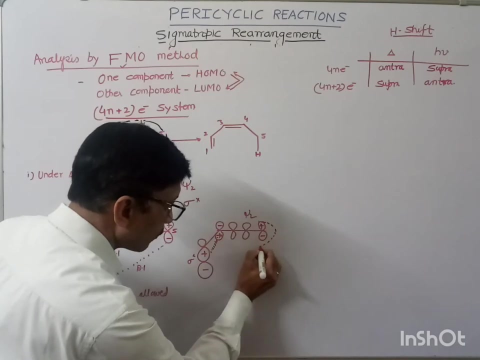 This is positive, This is negative. This is sigma star, This is our side 2. And if you will go for the entra means opposite loops should interact in a entra. So now this will interact to form bonding, But here this will interact to form a anti-bonding interaction. 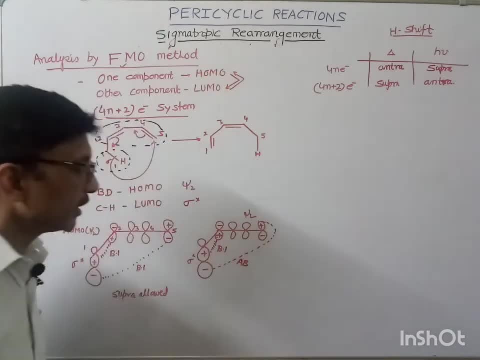 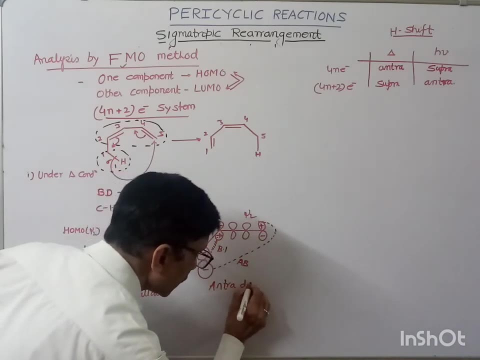 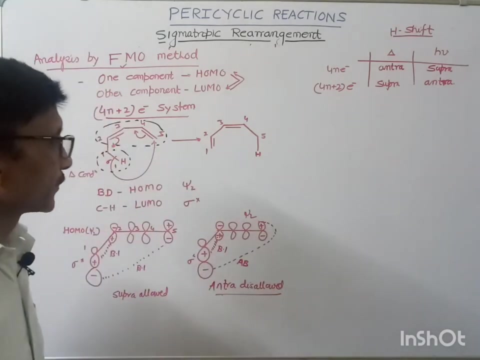 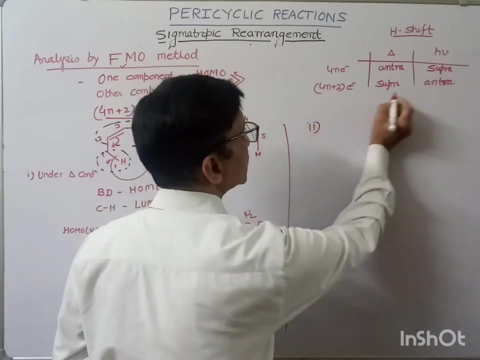 This is anti-bonding interaction, This is bonding. This is anti-bonding. This interaction is disallowed. So that is why entra Entra is disallowed. Entra is disallowed Here. Now, in a same manner we can prove for second case, that is here: 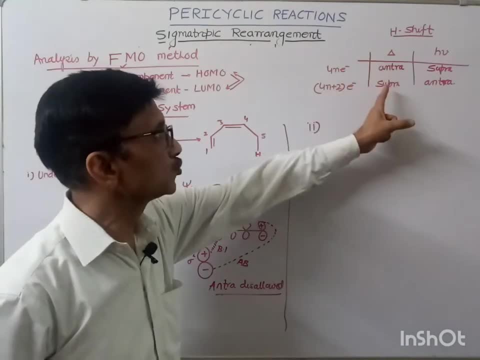 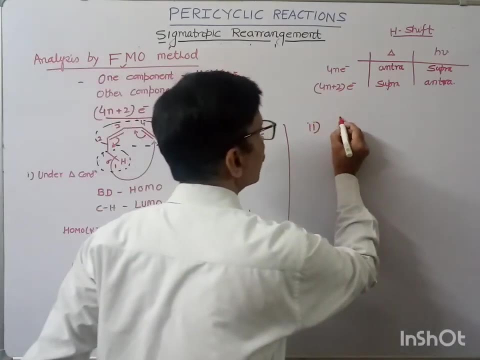 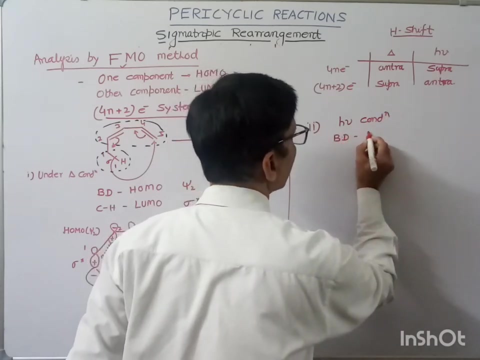 Entra what I have told you. under thermal condition, only supra is allowed. Only supra is allowed. Entra is not allowed. Now for thermal photochemical condition. Photochemical condition: The butadiene, Butadiene, homo Homo of butadiene, that becomes psi 3.. 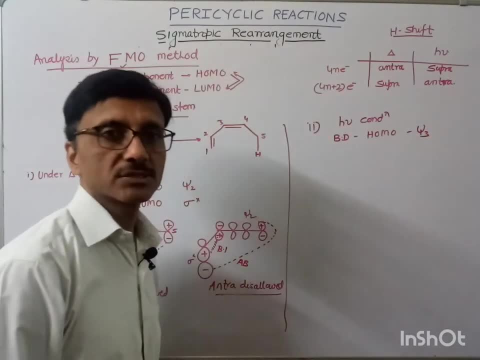 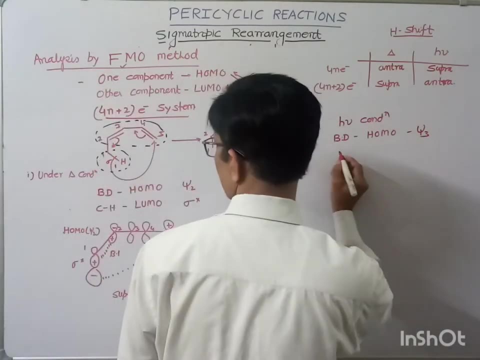 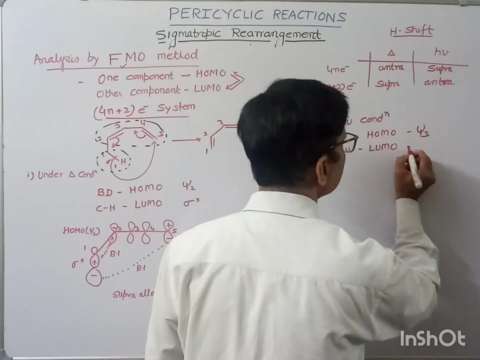 That becomes psi 3. already I have, when you, the lecture on this molecular orbitals And this homo lumo and the symmetries. already I have given the lectures. So C-H sigma bond, This is lumo And lumo for C-H sigma bond under photochemical condition, this will remain same, that is psi. 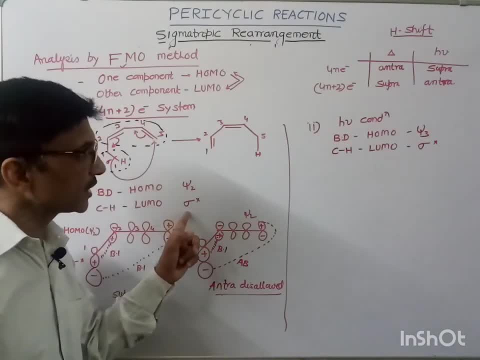 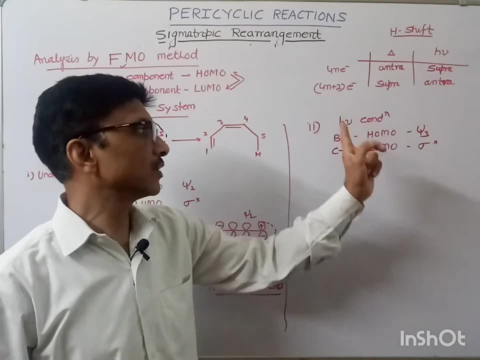 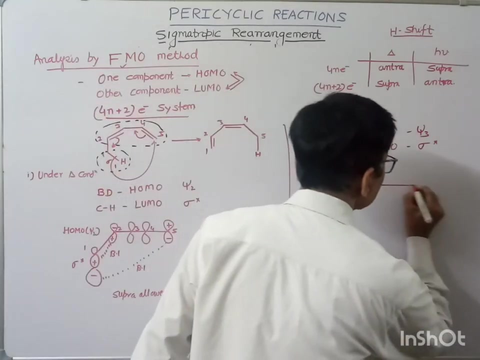 sigma star. So under photochemical condition lumo would be sigma star. Under thermal condition lumo is sigma star, And under photochemical condition also the lumo of C-H bond. that will remain the sigma star. Now, first of all for butadiene. these are the four orbitals of butadiene. 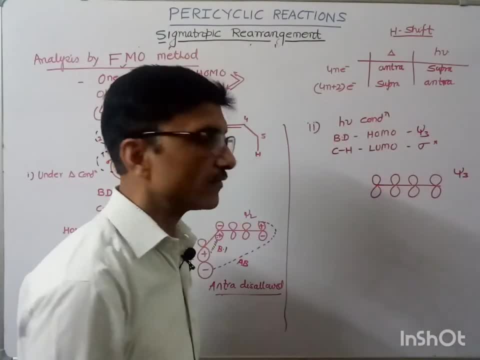 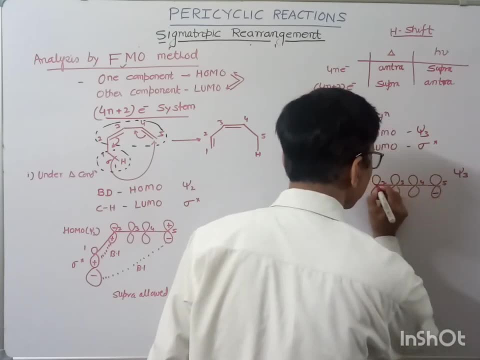 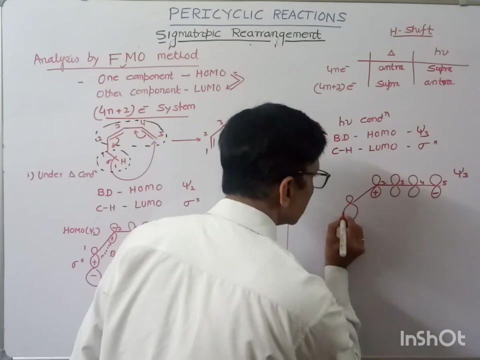 And psi 3, for psi 3, the end orbital that should have the opposite sign, plus, minus. And suppose this is fifth carbon, This is fourth carbon, This is third, This is second, And this second, This is hydrogen And this is, this bond, is the sigma star. 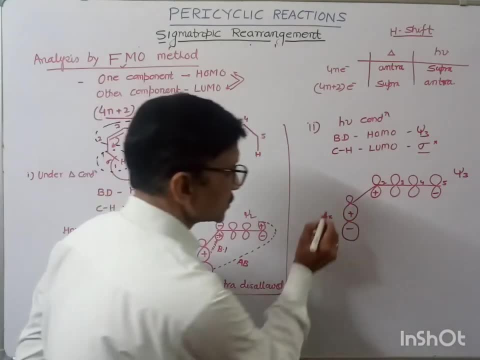 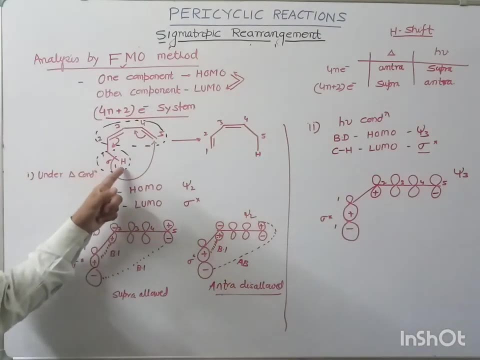 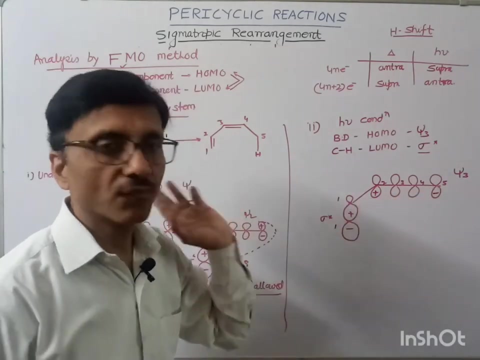 So for sigma star we should write plus minus. So this is our first carbon And this is attached to this first carbon is attached to the, this hydrogen, which is also given in the number 1.. So this breaks and 5, 1, 1, 5 bond. that should get formed. 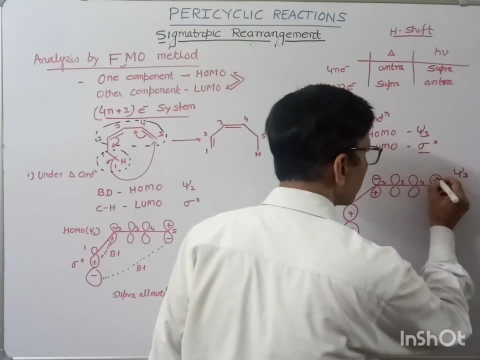 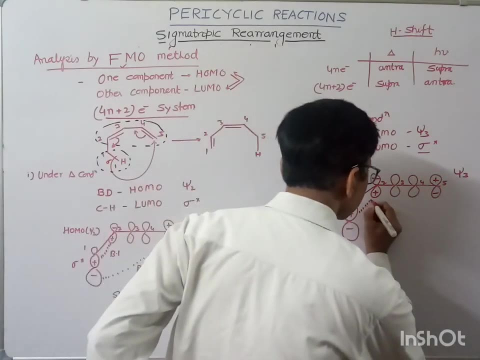 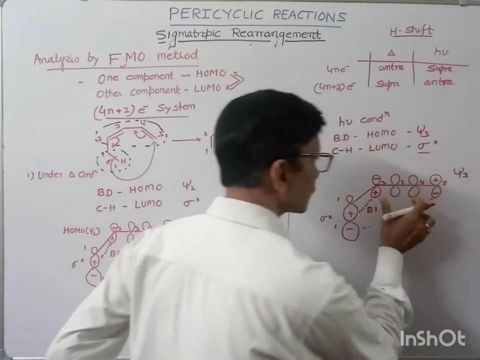 Now if it interact in a suprafacial manner, whether it is possible in a suprafacial manner. Let us see bonding interaction Here also in a suprafacial means. same side lobes interact. in a suprafacial interaction, same side lobe will interact. 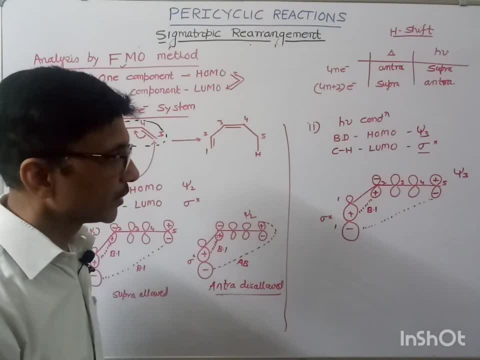 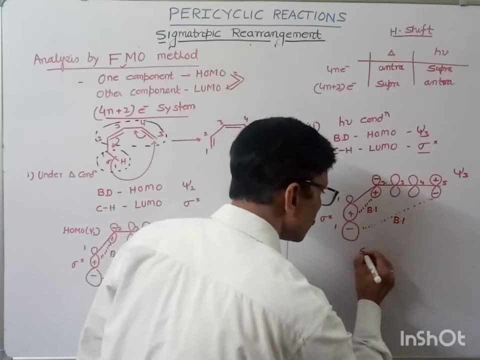 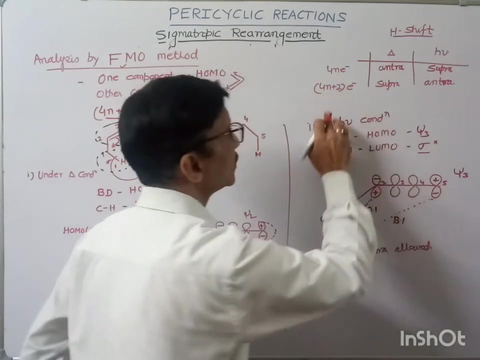 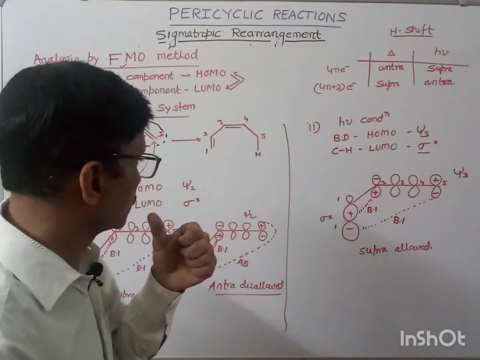 In an interfacial interaction, opposite side lobe interact. So what you can see, both are the bonding interaction. That is why. that is why this interaction supra is allowed over here in photochemical condition. In photochemical condition for 4n plus 2 electron system, the sorry, sorry, sorry. 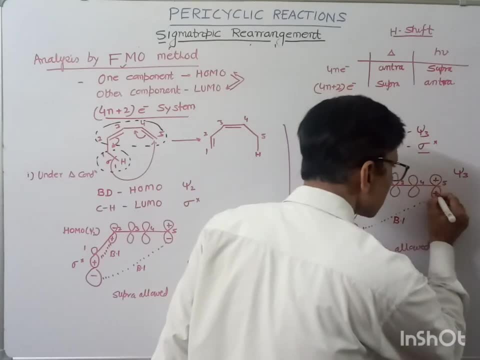 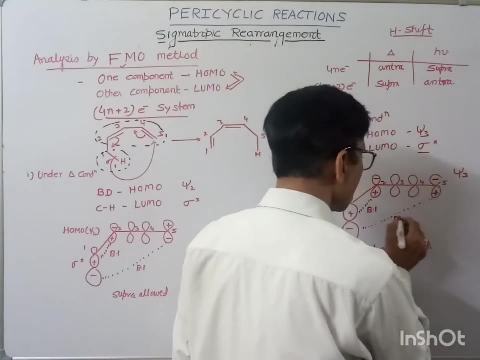 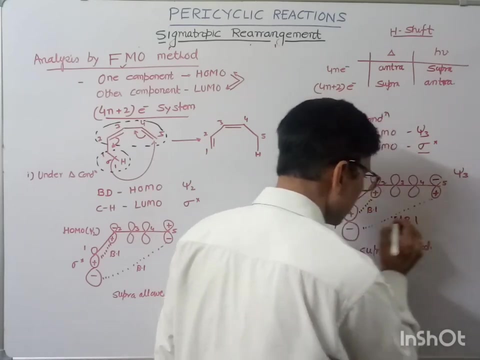 So this is actually plus psi 3.. Psi 3 means end orbital should have the same sign and this will be minus. Now, if you will see the suprafacial, then antibonding interaction is taking place over here. Antibonding interaction, and that is why supra is disallowed in this phase. 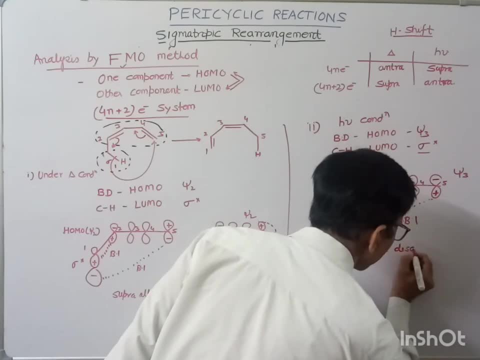 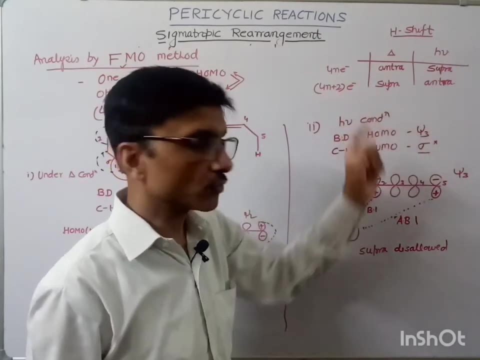 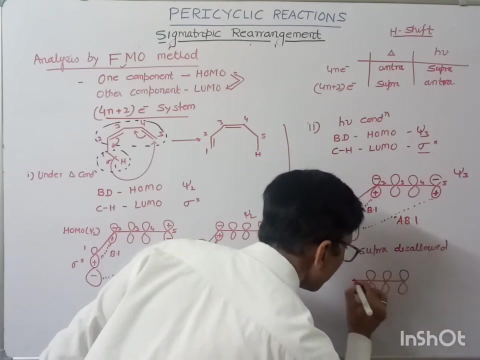 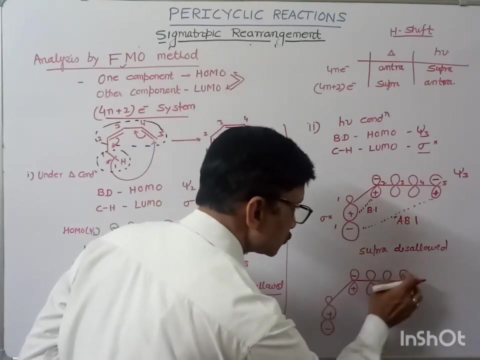 Supra is disallowed, Means entra should be allowed. Entra is allowed under photochemical condition for 4n plus 2 electron system. So now let us see for interfacial interaction. And orbital is having the same sign. Now interfacial interaction, these two lobes should interact. 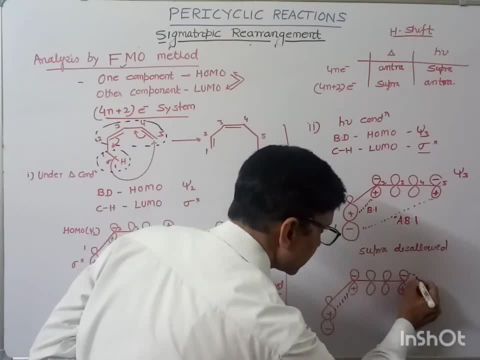 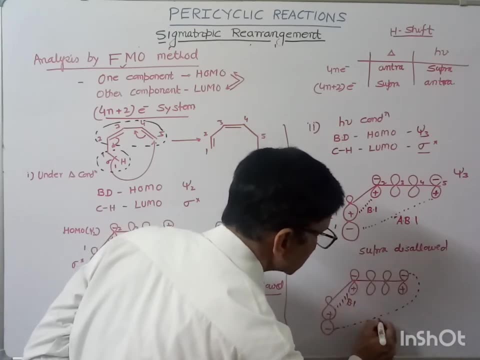 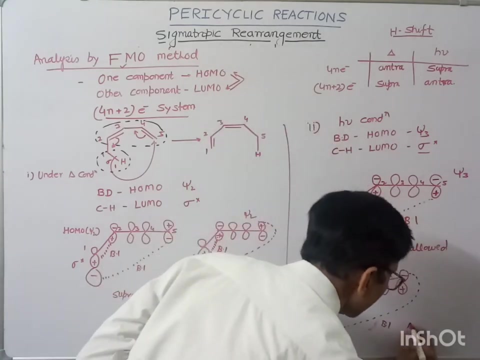 So these two lobes should interact. one is interacting with this one and another interacting with this one. So this is our bonding interaction and this is our antibonding interaction. Bonding interaction and bonding interaction. that is why entra entra is allowed. 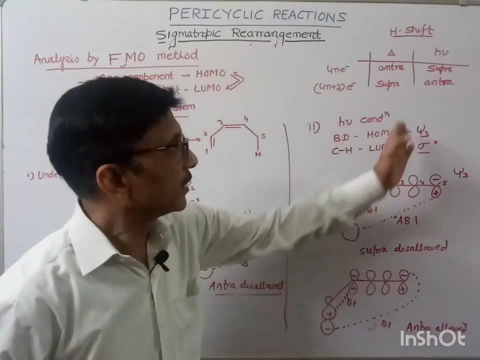 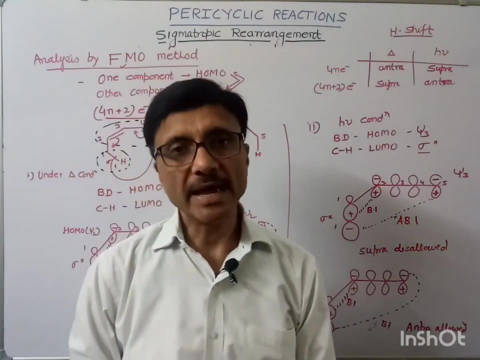 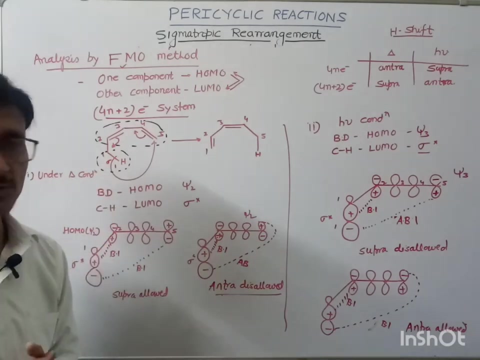 Entra is allowed. So this is thus. we have proved the, this sigmatropic rearrangement by FMO analysis. Now, in a same way we can prove for the alkyl shift, also in a same way, alkyl shift, that can be proved. 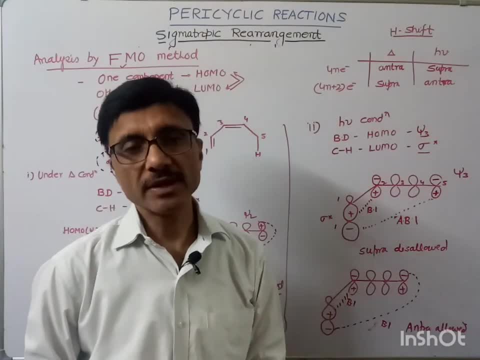 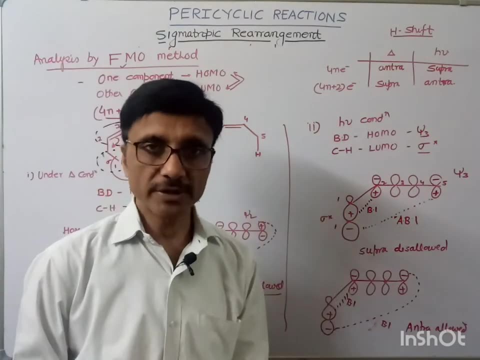 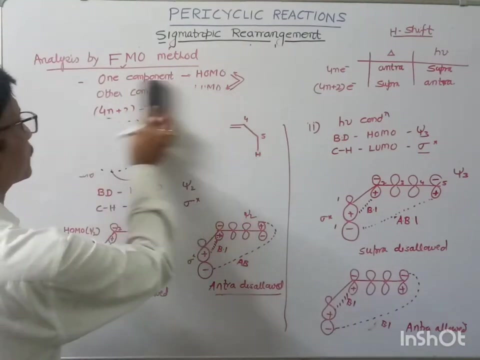 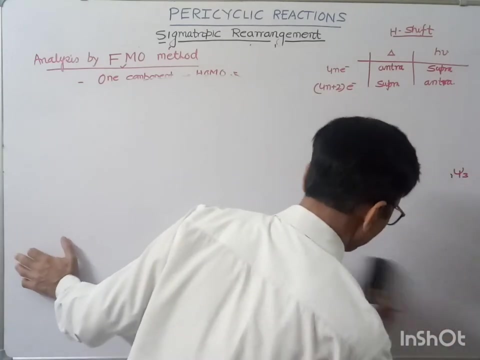 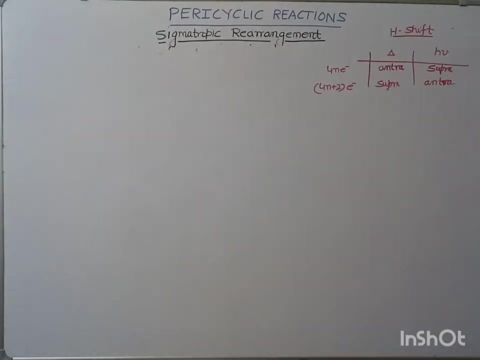 I have given the selection rule for the alkyl shift and analysis of this alkyl shift by the radical approach that I have already told you in my previous lecture. You may go through in that lecture Now. let us see few examples Now. if you see the example, then 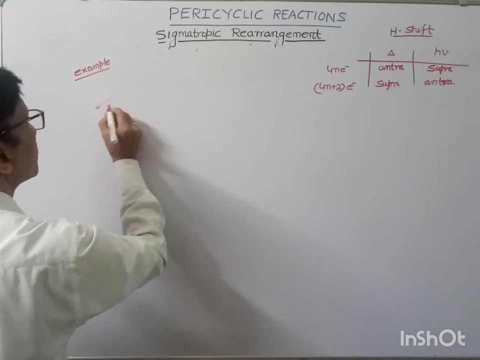 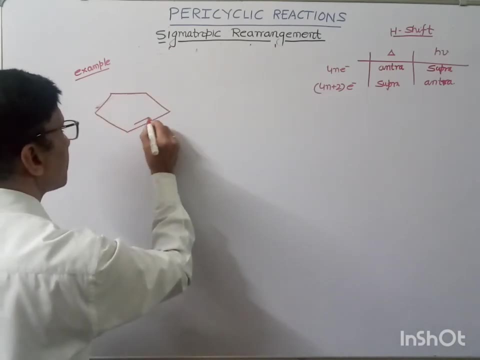 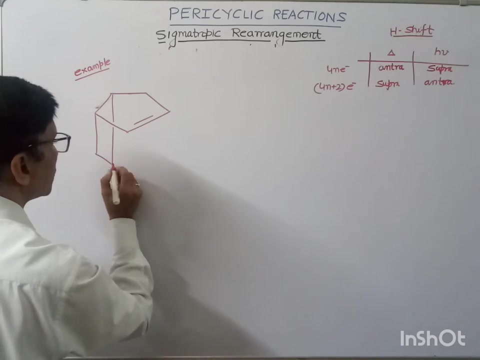 Now suppose, if you have, Let us see the Now. suppose you have, Now suppose you have, what should be the product of this reaction, what should be the product for this reaction? let us see this one now. first of all, what i have told you in such reaction in sigma tropic: 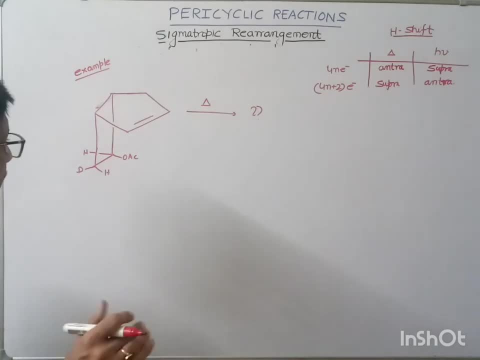 rearrangement. first of all, we should give the numbering and allylic carbon that should be given number one. so if this is one, this would be two and this is given number three. and now, from this first carbon, allylic carbon, the another, which is group or atom, is attached is: this is the another group. 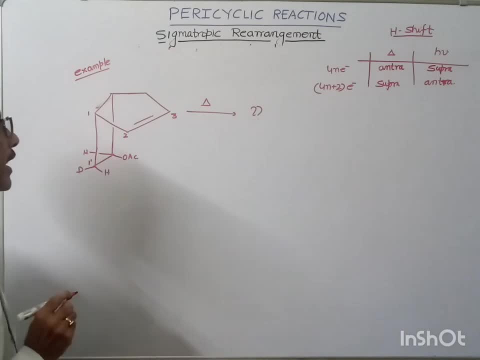 of atom which is attached- suppose i give it number one dash. and we know that in sigma topic, reaction one: one bond break and here the three. one bond should get formed, three one bond that should form now which one that should break over here. here this bond should break, this bond that should break and new bond that should be formed between one and three. 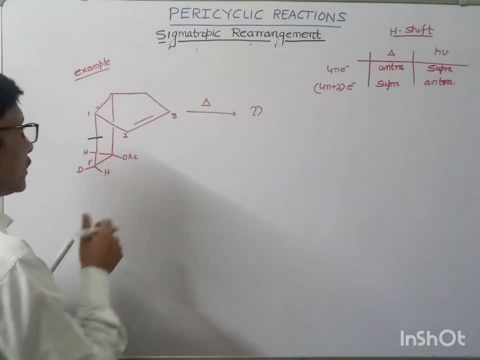 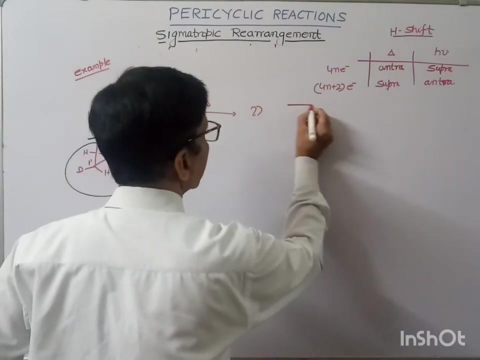 this one will get formed. so the how you can draw, how you can rotate it, this bond will rotate like this. so if this is formed, then here this buoyancy of carbon will get increased and now this bond, this sigma bond, break, and it will, it will form a new bond at this position. that is third position. okay now. so if you will write here, 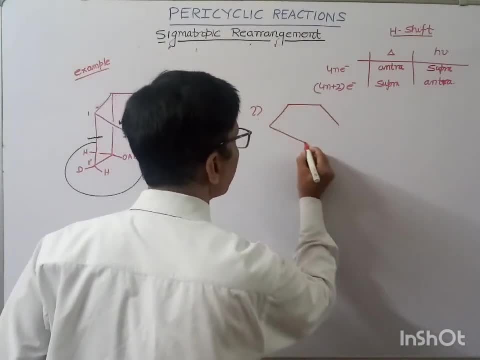 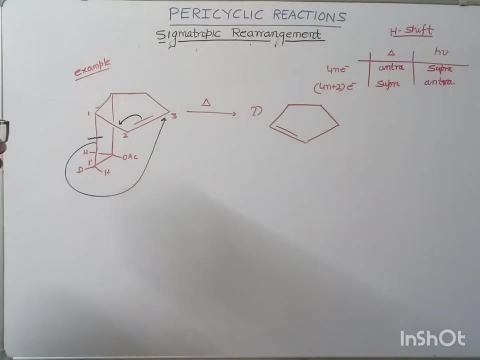 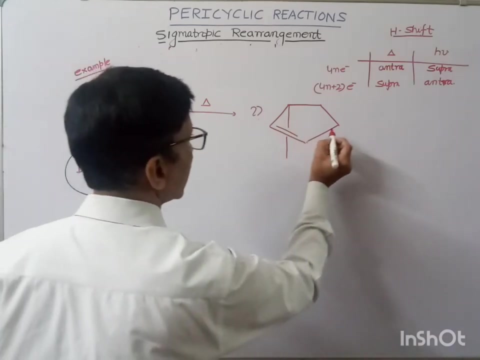 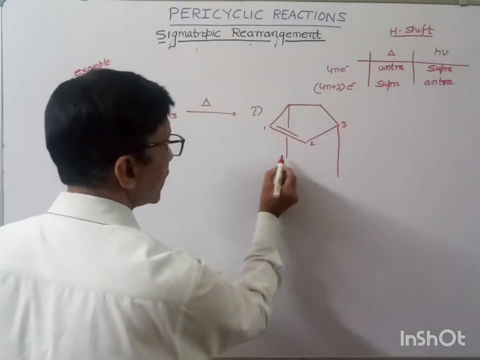 then now. so new bond is formed between first and new pi bond is formed between first and second, and this one one dash is broken down and this remains same. this remains same and new bond is formed over here. that is third, this is second and this is first suppose. 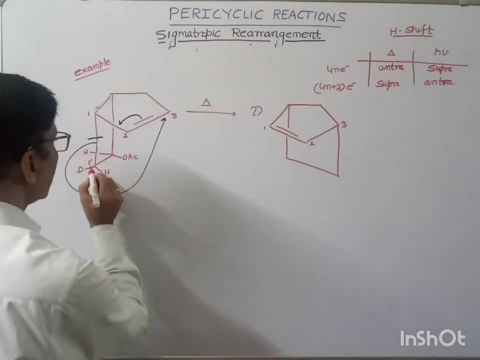 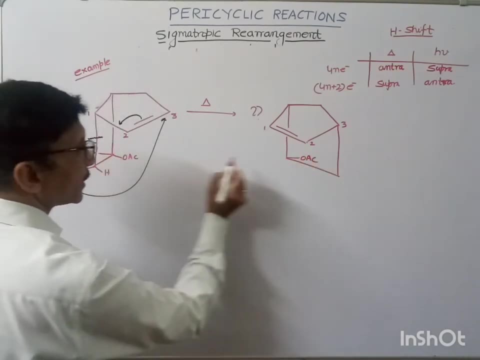 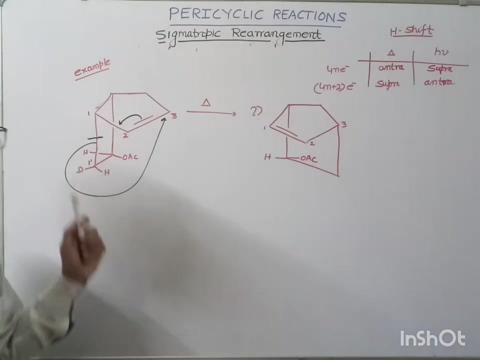 and new one. you will see, this is a new one which is formed, and here this is your oec acetate group is present over here and the hydrogen is present over here. now, what about the stereochemistry now kind of shift? this is not the hydrogen shift, this alkyl group is shifting. 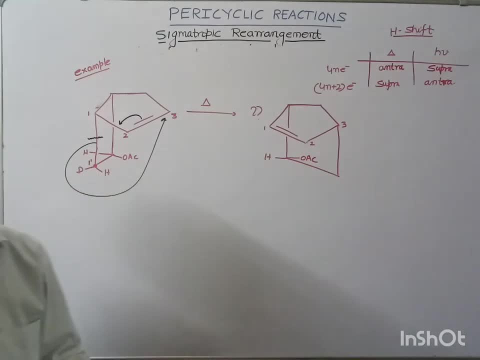 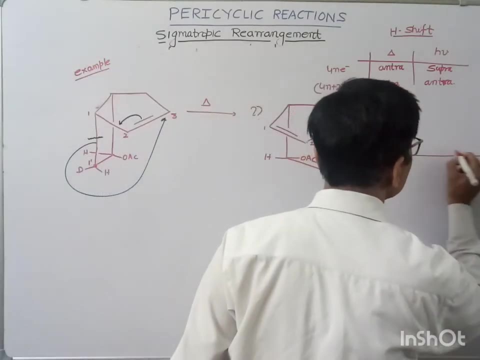 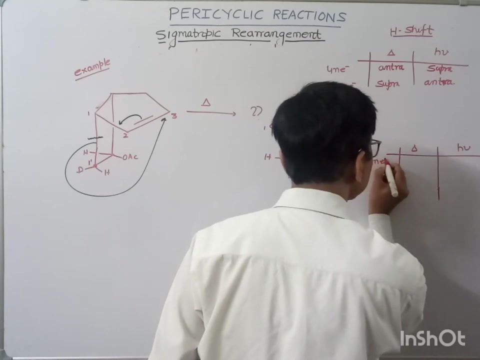 the shifting of alkyl group is taking place and for alkyl shift, i have already given you the rule. i have already given you the rule. what was the rule for the alkyl shift or for an electron system and for 4n plus 2 electron system? the rule that i have told you. 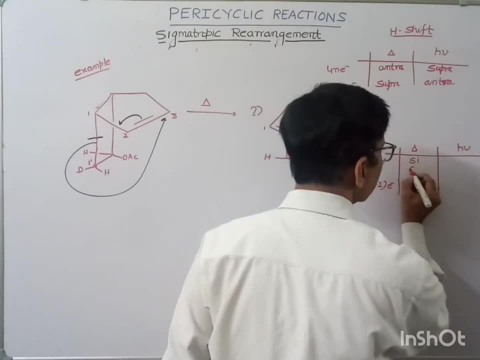 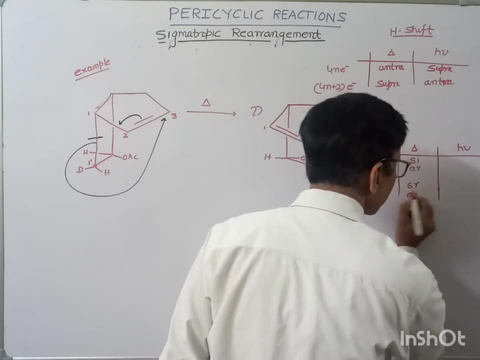 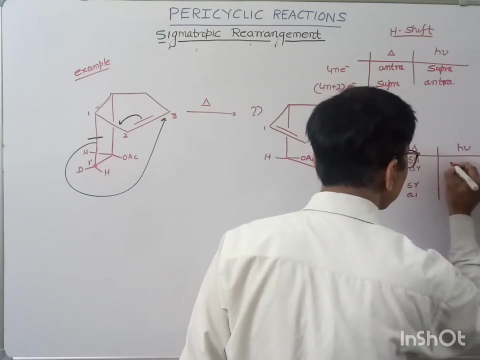 is that for alkyl shift, for this alkyl shift, we have to write after this, and the rule is: super facial with inversion or interficial with retention, or super facial with retention, interficial with inversion, and write down diagonally in a same manner. so this is the rule. 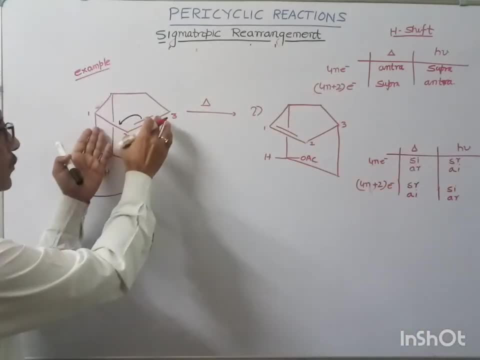 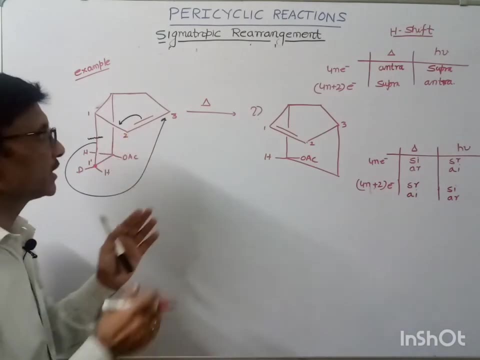 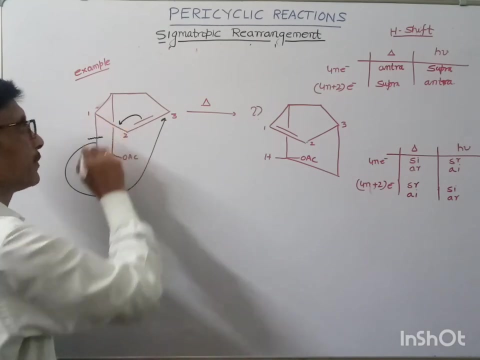 that i i told you for alkyl shift. this is the rule. now this is an example of In this reaction, these two electrons, they are participating in the reaction, and this sigma bond electron, they are participating in this reaction. So this is an example of 4N electron system. 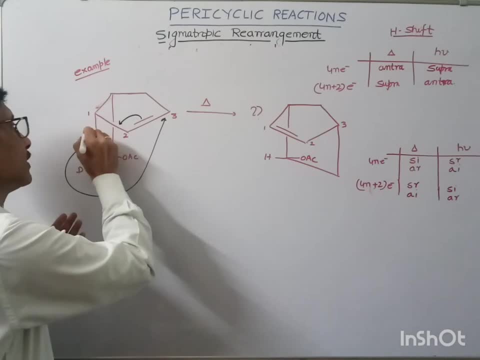 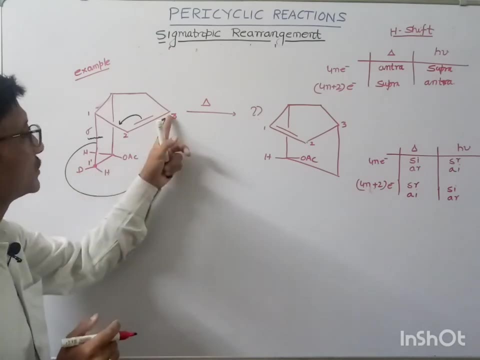 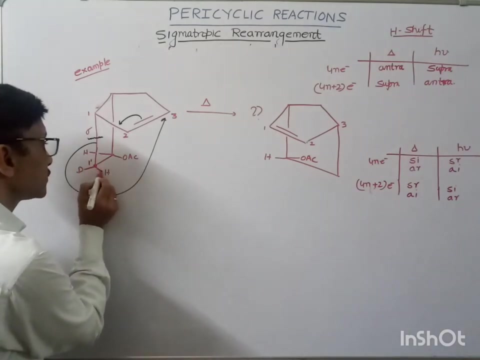 This pi bond is involved in this reaction and this sigma bond is involved in this reaction. CC sigma bond is involved in this reaction And shift is the Lp shift which is shifted to the third position. So here this is shifted Now. so what should be the stereochemistry of this substituent which are present on this carbon? 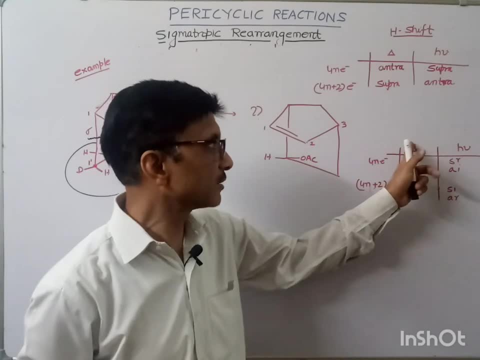 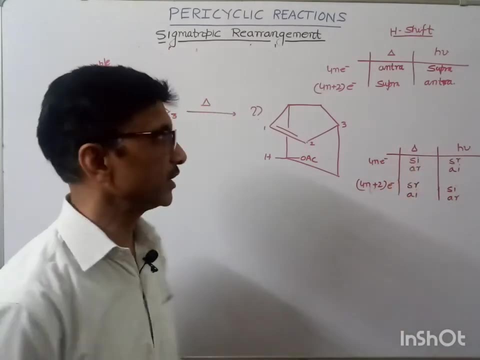 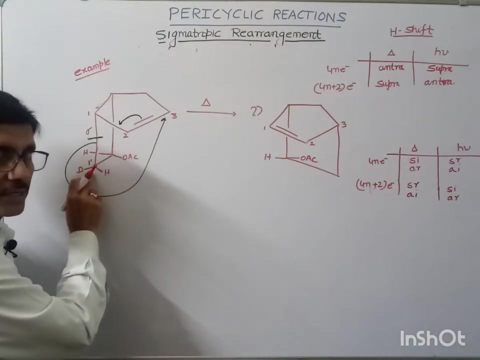 So because this is 4N electron system under thermal condition, under thermal condition superficially, it should interact with the inversion of configuration. So same side superficially, but the stereochemistry of this will get inversion, So inversion of this alkyl group that will take place over here. 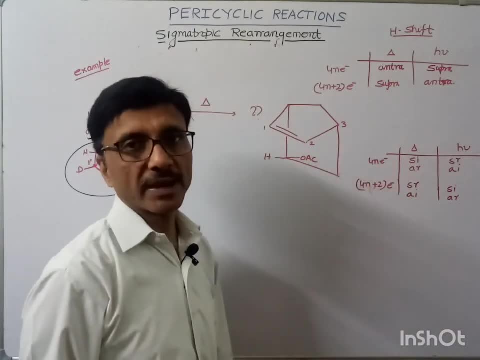 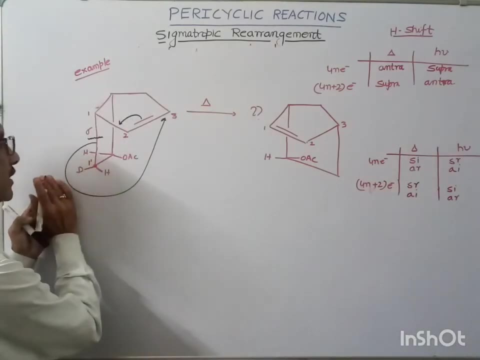 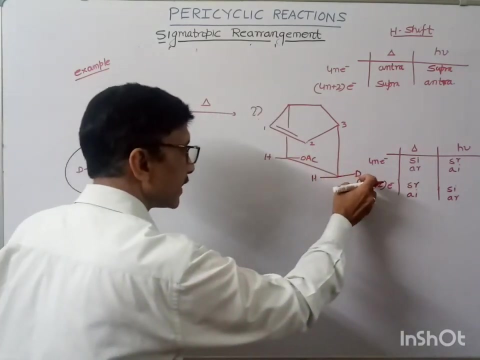 After suprafacial migration. after suprafacial migration inversion that should place Here D deuterium is on the left side. That is why it should go on the this side and this will go on the this side. So it will go on the right side and hydrogen is going on the left side. 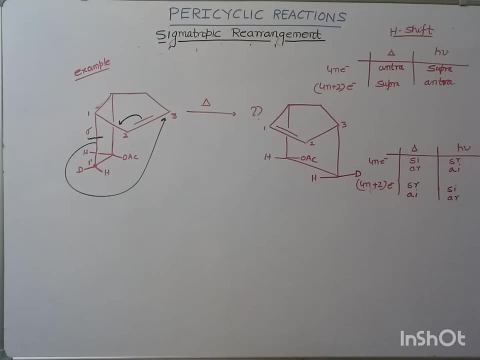 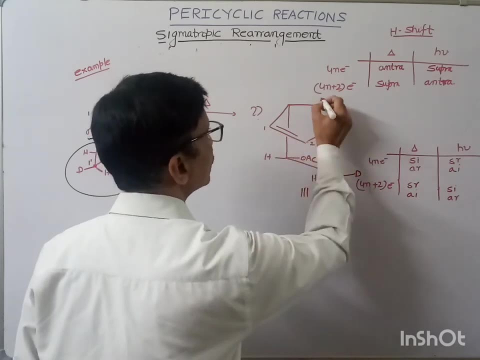 So this would be the case for this one. Now we can also show it in another manner. We can show it. Suppose this is 1., 2., 3.. If it is 4., 5.. And suppose this is 6.. 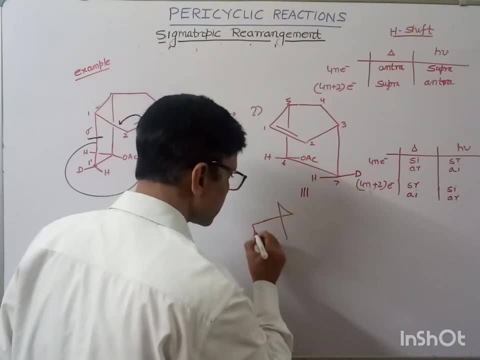 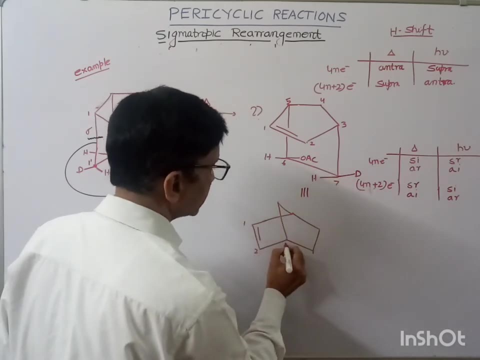 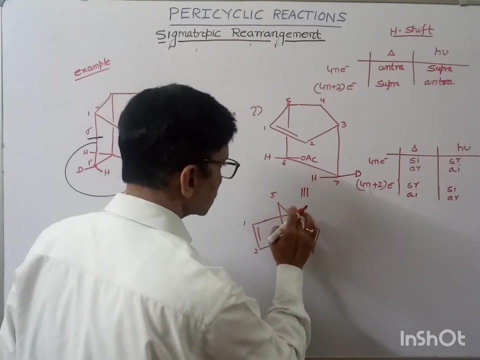 This is 7.. And we may show it in another manner, like this: You will see, And suppose, this is our first carbon, second carbon, And this is third, one, fourth and fifth, And from fifth, this is first, second. 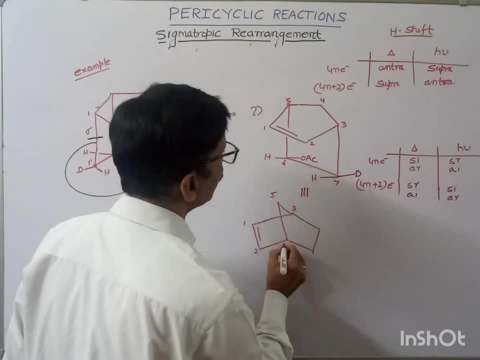 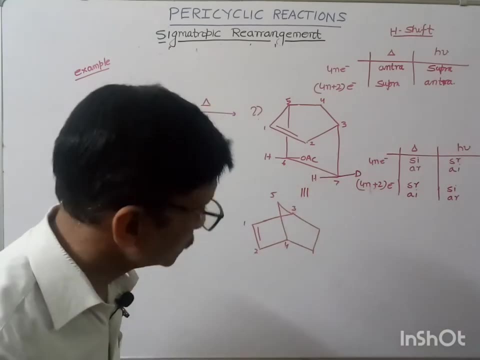 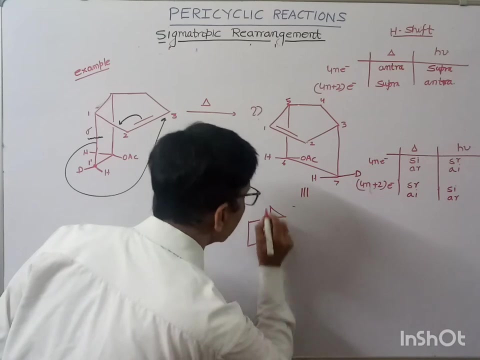 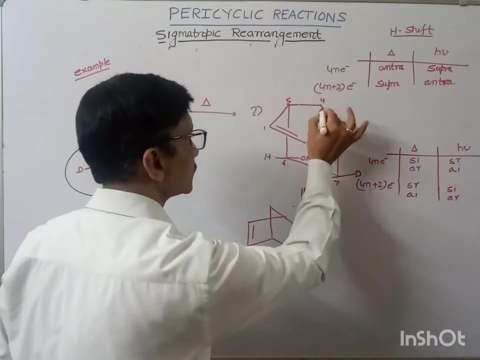 And suppose this is third, And this is fourth And this is fifth one. So we may show it in this manner: This one, This is our first, second one And here fourth, This is the fourth one, This is fifth one. 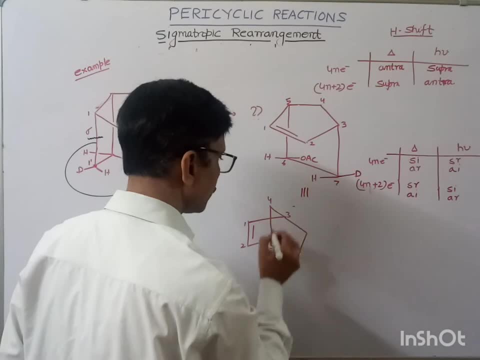 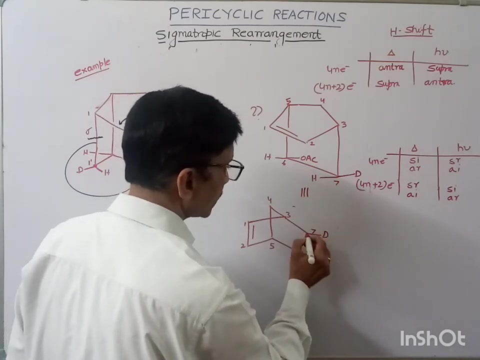 And this is our first, second, third, fourth And this is our fifth. From fifth, sixth carbon is attached And from sixth, seventh carbon is attached. Seven is attached to third one. Seven is attached to third one. Now, at seventh carbon you may see, this is D and deuterium and H. 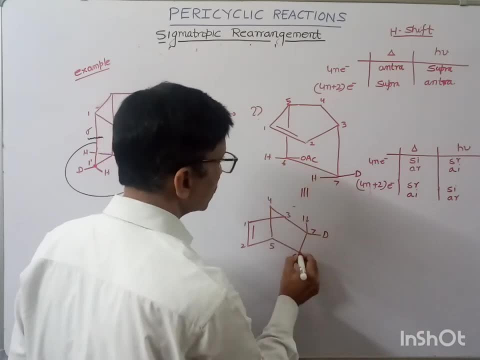 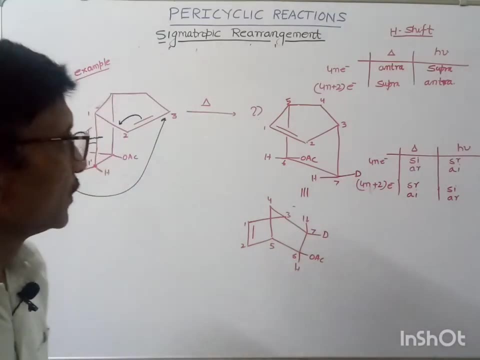 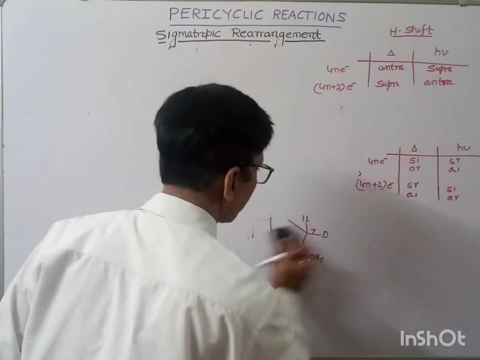 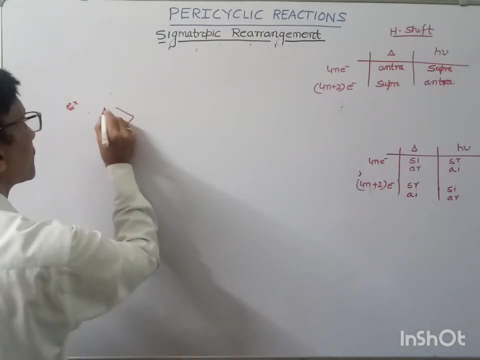 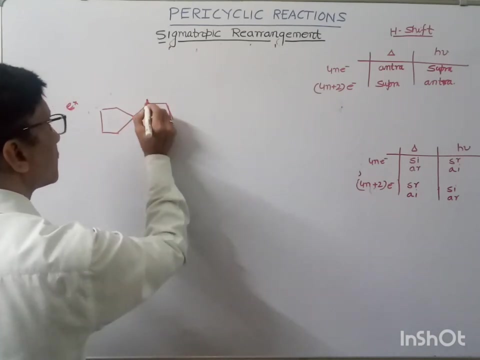 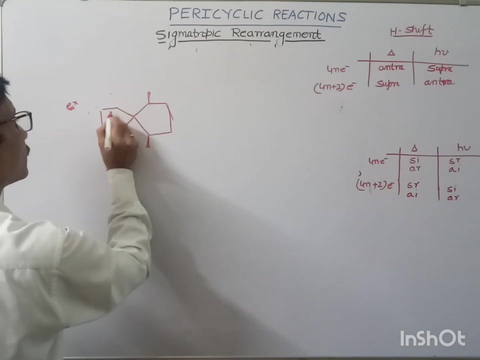 And here also at this one. this one is C And this is C, So you may write it in this form also. Now, let us see the another problem. Now, let us see the another problem. Okay, Now. so here, what should be the product of this reaction under thermal condition? 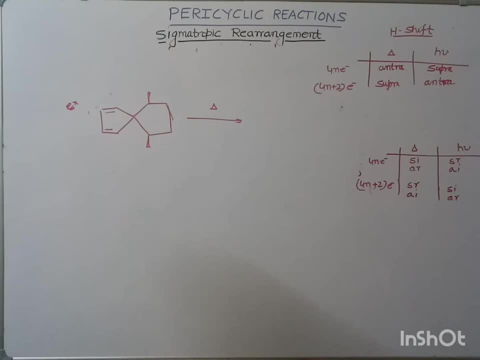 Now under thermal condition, if you will see the product, then first of all we should give the numbering, The allylic carbon, that should give a number 1.. So if this is given, number 1,, this is 2, this is 3,, 4 and 5, and from first another. 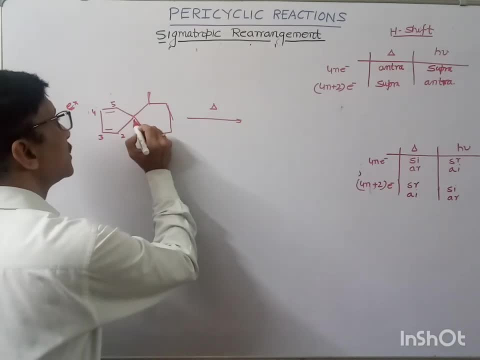 atom, carbon atom, is attached. so either this may be given- suppose I have given number 1 dash- or this may also be given 1 number 1 dash. Now which bond breaks in sematopic reaction? which bond breaks 1, 1, that breaks. 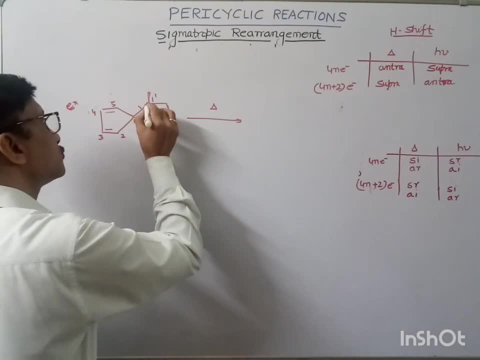 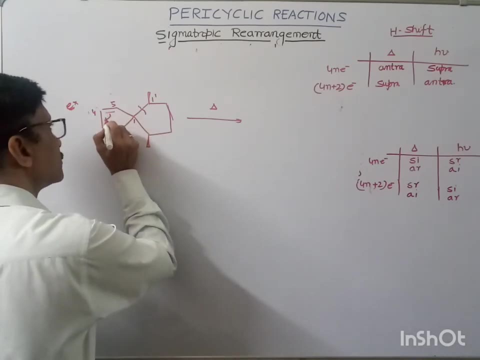 1, 1 breaks and it should attach to the 5th position. So how? After getting this energy, after getting this energy, so the shift of these pi electron will get start. and this here, the valency of this carbon is increased, this bond will. 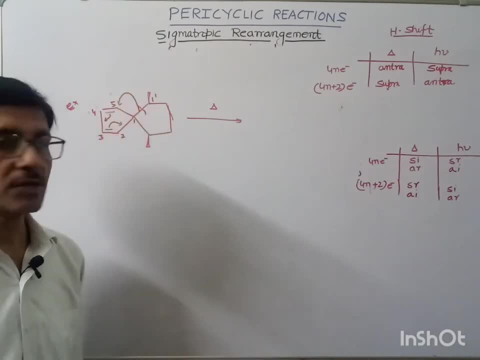 break and this will go over the This unsaturated part. From saturated to unsaturated, the shift takes place. So, as you can see here, this bond has broken down. This bond has broken down. This is broken and new bond is formed between 5 and 1 dash. 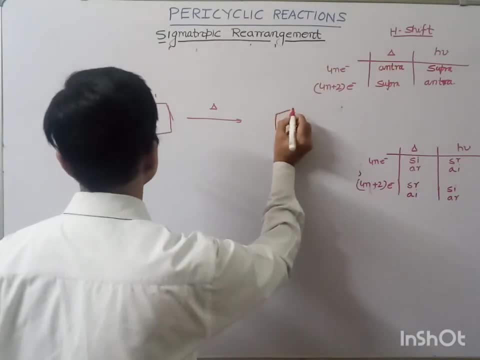 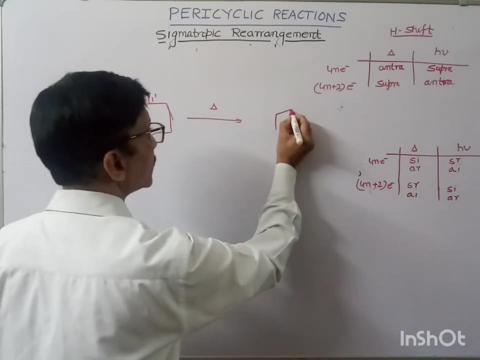 So what you can see this is, and a 6-member ring is formed: 1,, 2,, 3,, 4,, 5, 6-member ring is formed over here. So this is the 6-member ring. 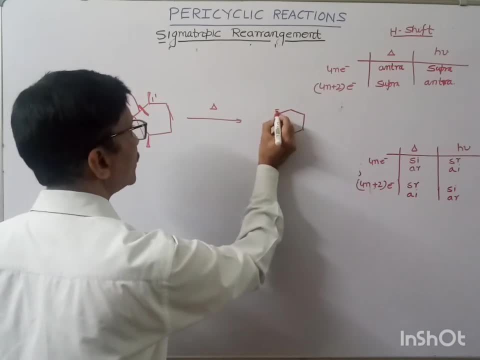 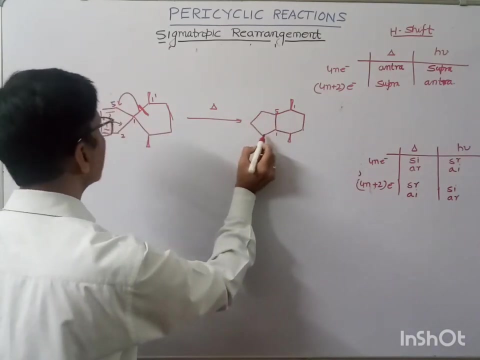 And suppose this is our 1, and this is 5 and this is the 1 dash and this 1 dash, our, this methyl group is present And now from 5th, you may see this 4th is formed, this is 3,, this is 2,, like this: 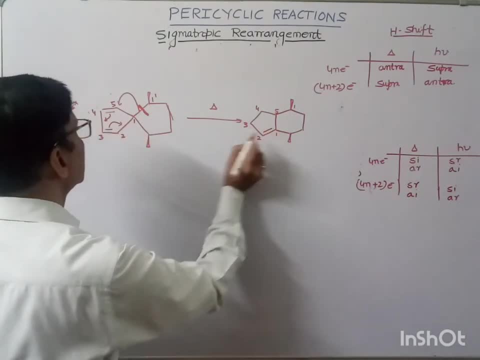 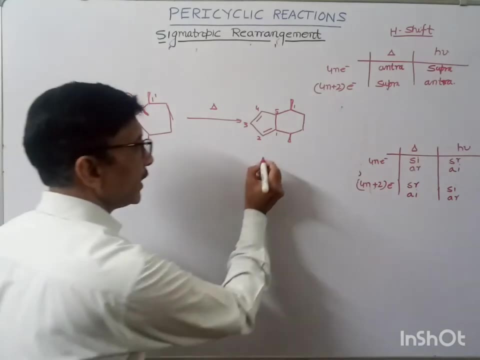 Now a new bond is formed between 1st and 2nd And another bond is formed between 4th and 3rd. This could be the case Now, in next, what may happen? Now again, we may give the numbering. 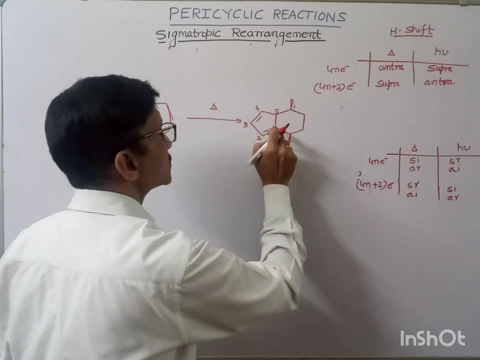 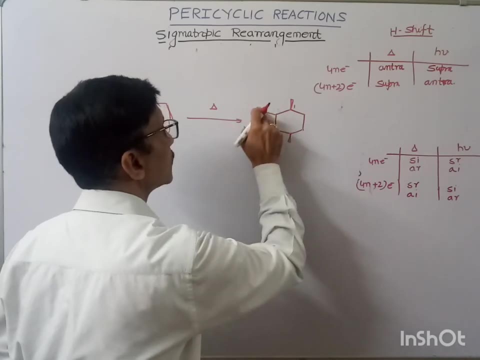 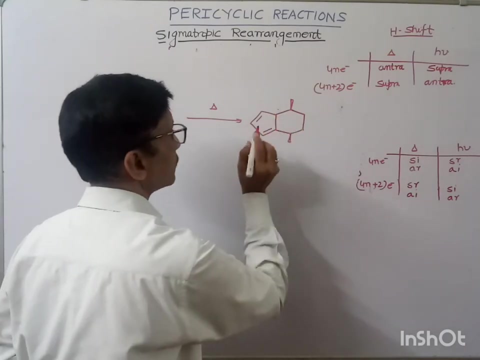 Again, we may give the numbering And suppose, suppose here one of the suppose, what I should give. So this is the form, This is the compound which is formed. And now suppose, this is the allylic carbon. 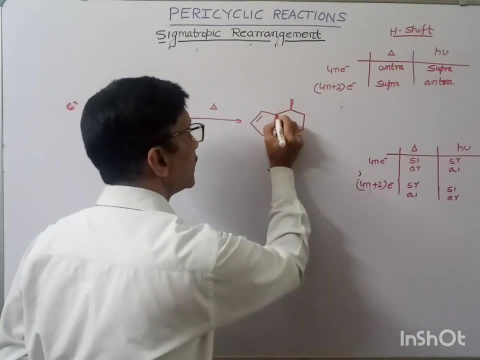 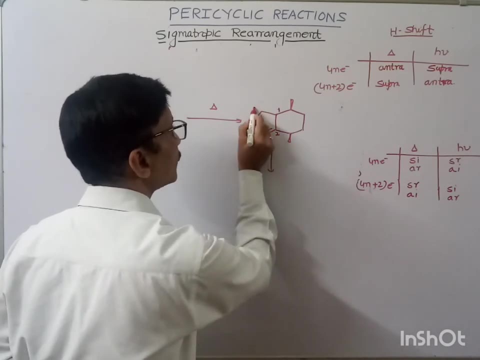 Again, we should see for the allylic carbon. We may see for the allylic carbon And this is the allylic carbon and that should be given the number 1 and this is 2, this is 3,, 4, 5.. 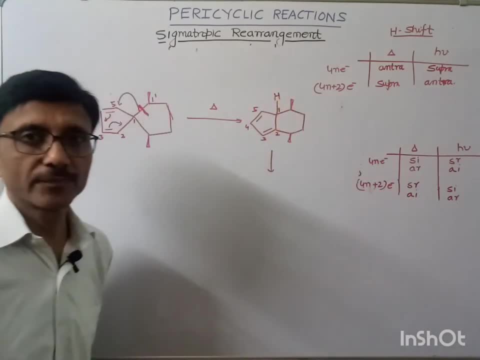 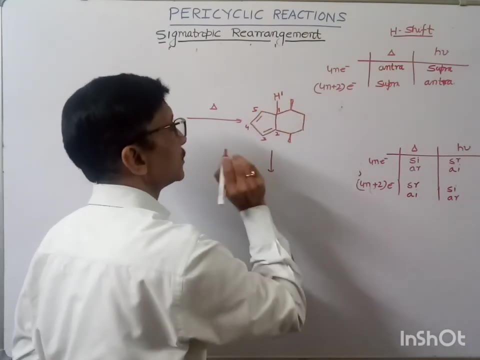 And from this allylic carbon you may see one of the hydrogen is present And this hydrogen, the atom attached to this allylic carbon, is also given number 1.. Okay, So this 1, 1 bond will break again. 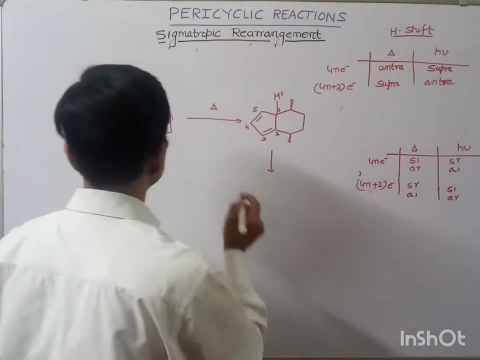 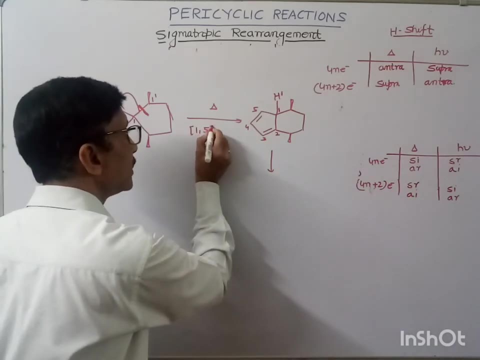 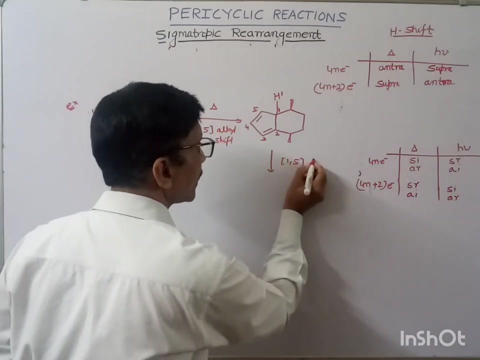 Again, sigma topic: hydrogen shift will take place. So here sigma 1, 5.. 1, 5, alkyl shift. here you can see 1, 5, alkyl shift has taken place And here 1, 5,. 1, 5, hydrogen shift will takes place over here. 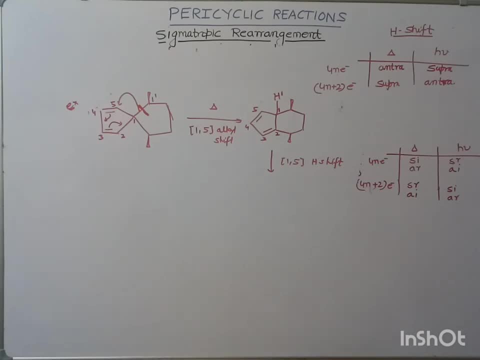 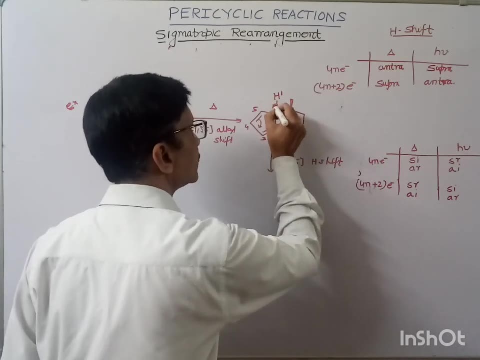 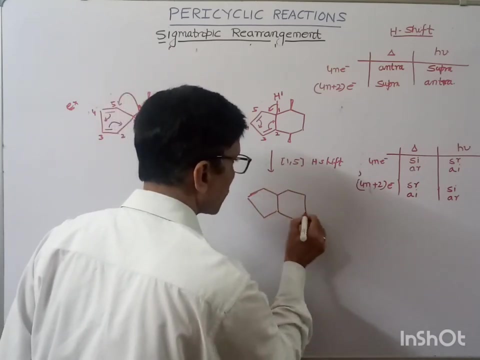 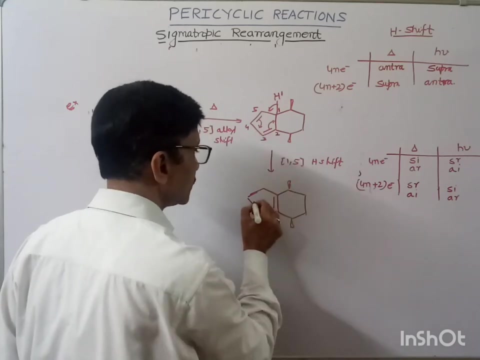 Hydrogen shift will takes place over here Now, so it will shift with this, bond will break and after this, what you will get, this will shift at over this place And finally, so now here, double bond, this double bond, now hydrogen is shifted at this. 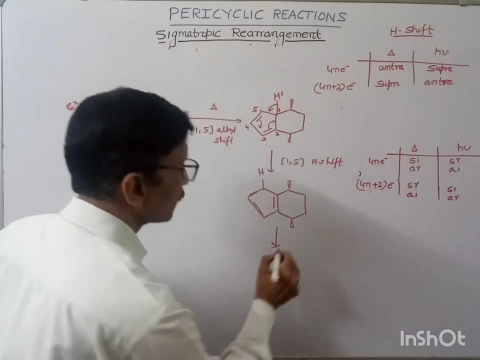 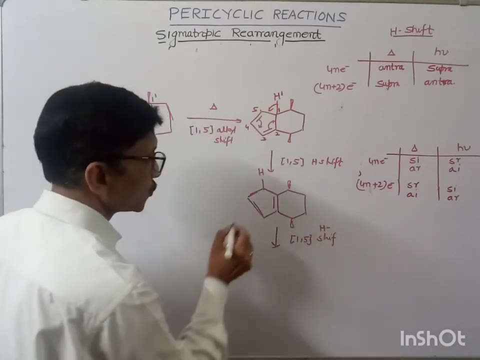 place. Now, again we may see: 1, 5 hydrogen shift is possible. 1, 5 hydrogen shift is possible, So again we may give: this is our allylic carbon, So this is 1, 5..